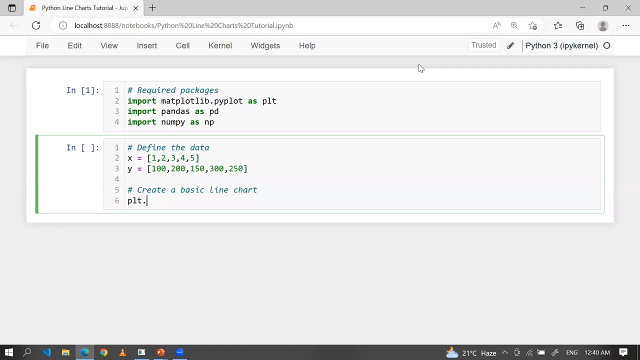 Okay, So simple. PLT dot plot. If you are writing plot, it means you are going to create a line chart. Now, simple again. you can supply the title, as we have seen in the last session. So basic line chart, guys, and PLT dot y x label. All right, So let's say this is the month and PLT dot y label. And, for an example, 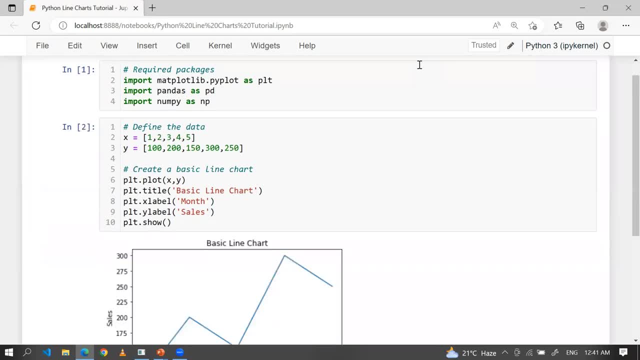 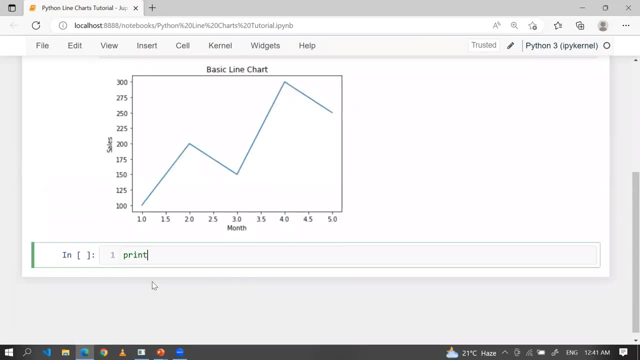 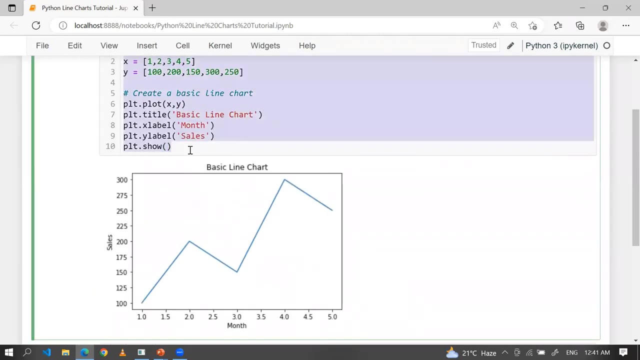 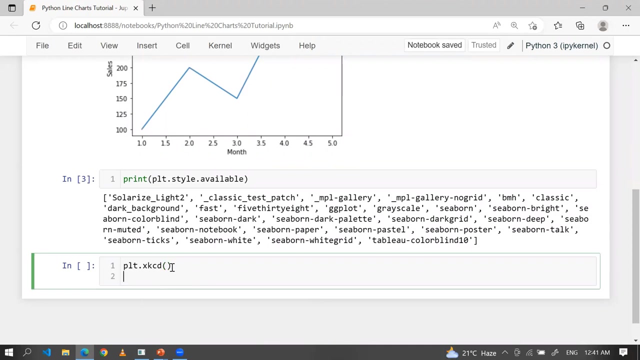 sales and PLT dot show. Okay, So it is very easy to do that. And, guys, in the last session I told you let's say what kind of style we have. So these are the styles. Apart from these styles, you can use one more style as well. So that style name is PLT dot xkcd. Okay, Now let me, you know, paste this. So look at this just like a handwritten line chart, All right. 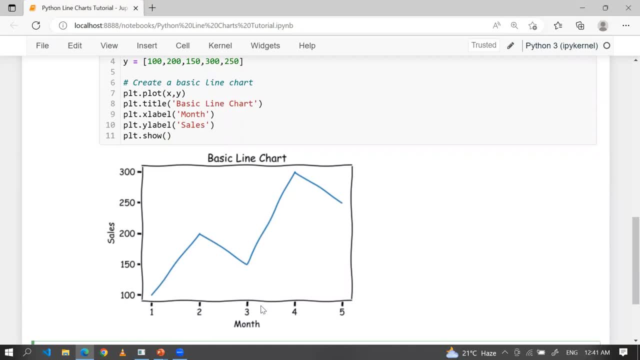 in case guys, can you see here? so this is the month one, two, three, four, and this is fluctuating my data based on my sales. so here, if I want the connector, okay, or maybe you know some market. so what can I do here? so simple, I have to copy this. 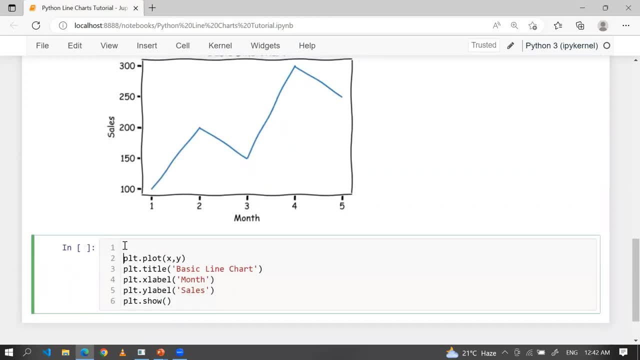 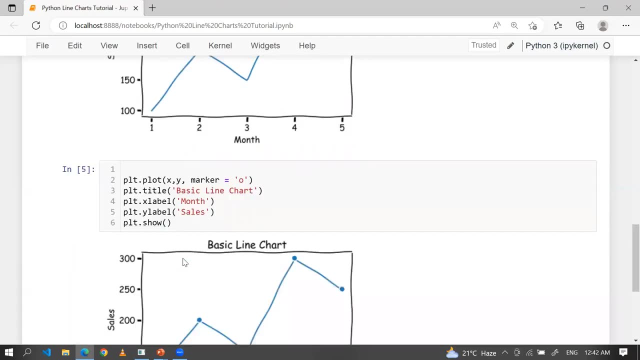 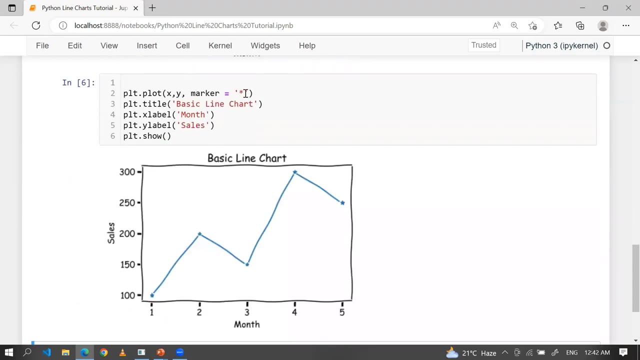 code, and here I can use X, comma, Y, and I want marker in the form of O shape. so look at this. okay, so these are the connectors. in case you want to change with a strict, so you can go with a Streg or than or less than sign, so you can use it. so now I am going to change line. 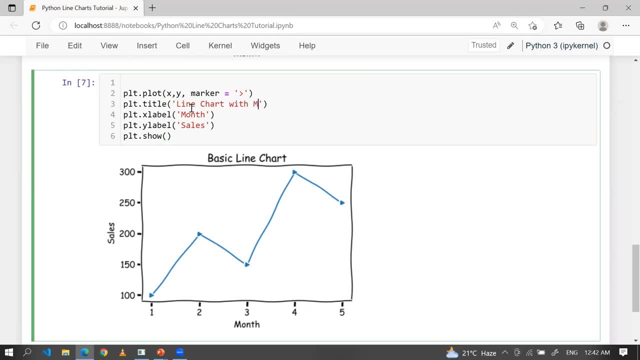 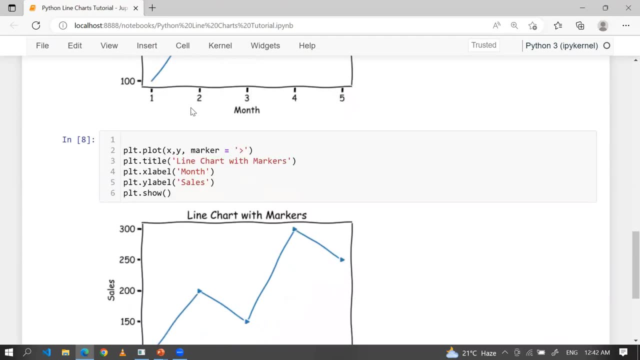 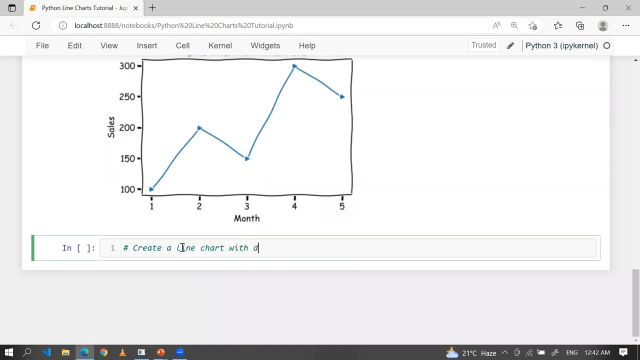 chart. okay, with markers. look at this. alright now. similarly, in case you want to supply that to line chart, okay, now, guys, what I am doing here: create a line chart. line chart with different line style, all right. so what can i do here? let's say, plt dot plot. 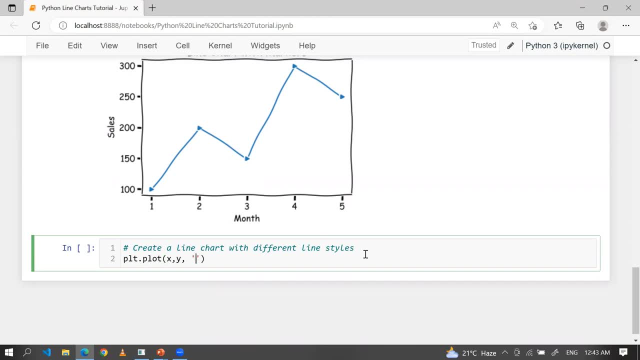 x axis, y axis, and here i am taking the o shape, let's say as a marker, and the color i want red, and, guys, the line width. line width, i want, let's say two, and i want to supply the label, right, so let's say line one, whatever line one. apart from this, one more line i am also going to. 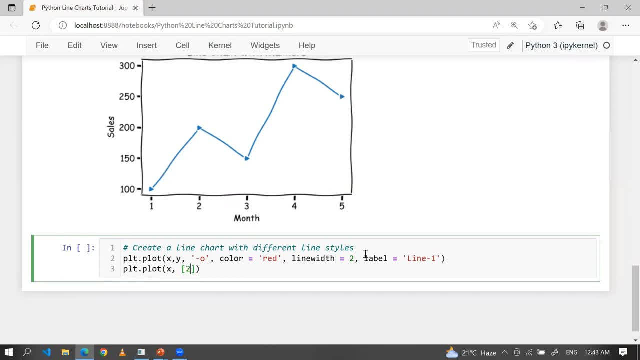 create x and i don't have y, so i am going to change my y. let's say with some you know the random numbers, so, for an example, 250 and 200 and let's say 150, right, so you can change accordingly. and i want the line style you know, like this and the color of this, this, that line, guys, i want blue. 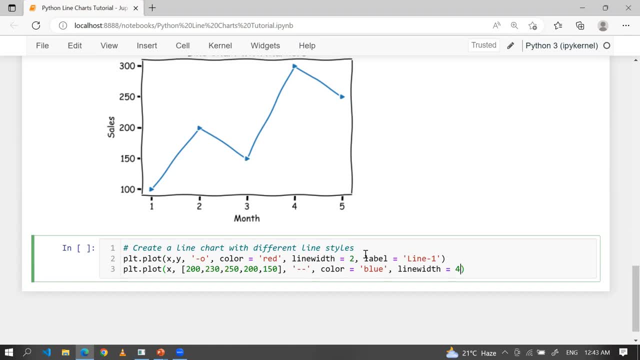 and i want to change the line width equal to four, and here the label, uh, equal to guys. i want line number as two, okay, and in case, if i want to supply the title, so what can i do? here? line chart with different line style: okay, whatever, right, and here plt dot x label, so let's say month, and here p. 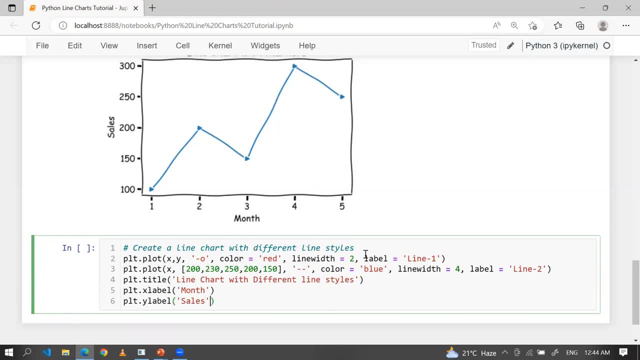 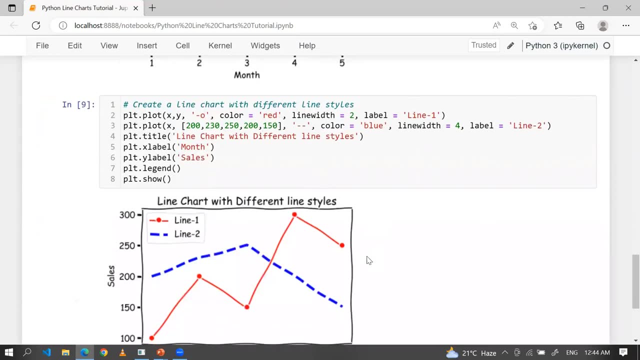 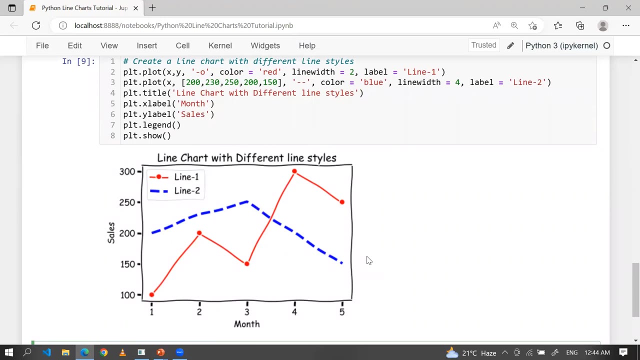 l t dot y label. i want sales, i want legend also. so, guys, this is legend and plt dot show. so look at this. okay, so that's how you can create a the line chart with the combination of two lines. all right, guys, so this is very easy to do that, in case you want to the you know grid line. so 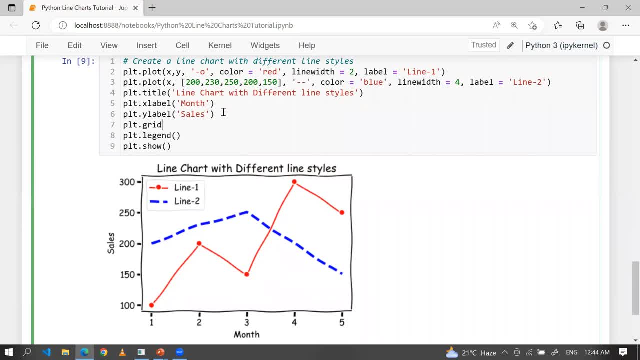 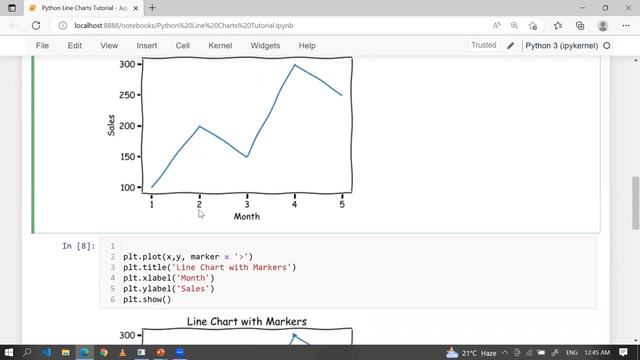 simple. you can use here plt dot grid and here you can use the parameters: true, i want the legend, i want grid line. plt dot grid and go true, all right. so, guys, right now the grid line is not swaying because it is not the part of this style which we have used: x, k, cd. all right so. 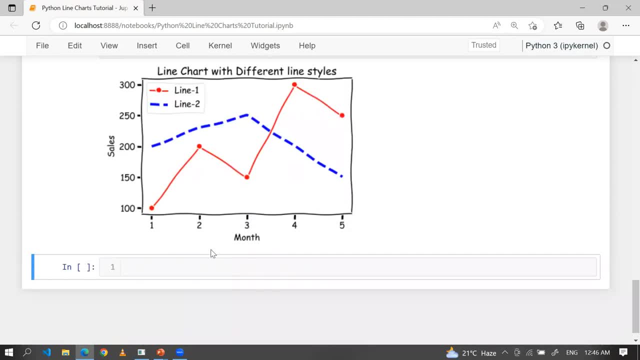 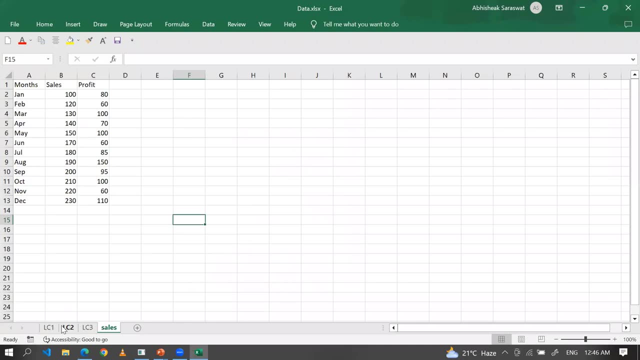 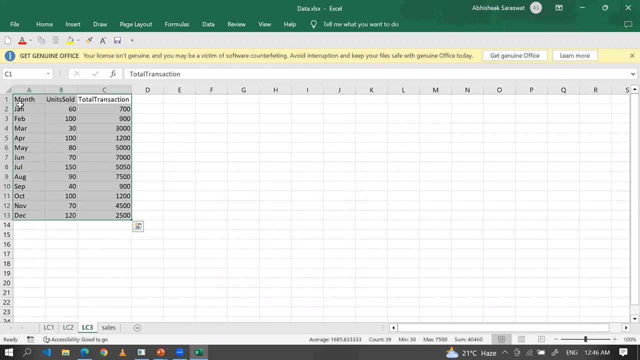 let me ignore this. and guys, uh, let's say, if i want to create the line chart based on the data, okay, so let me show you this data set. okay, so in this data set i have you know guys, you know category and right, i have month by sales and reason why sales and i have this data unit sold in total transaction. 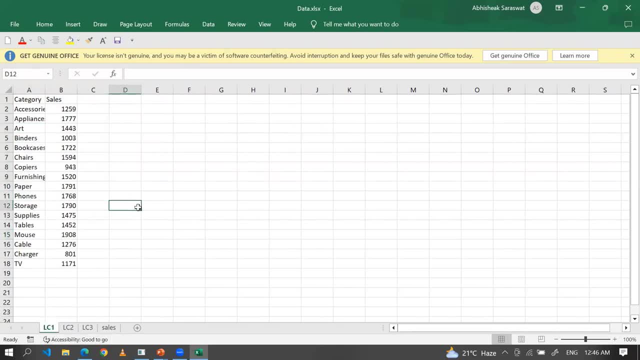 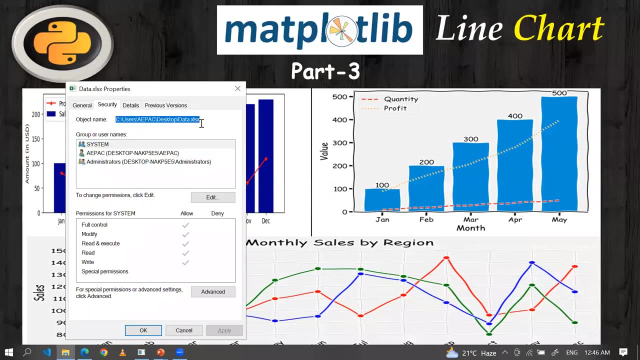 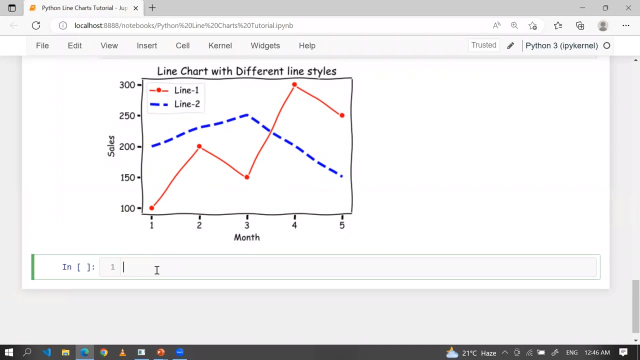 and i have this particular sales. okay, so i have some basic data set. okay, so, based based on this data set, guys, i want to create the chart. so let me take a path of this particular file. let's say this one, and here what i'm doing, so d, f, not df. or i can use guys let's say sales equal to pd, dot, read excel. 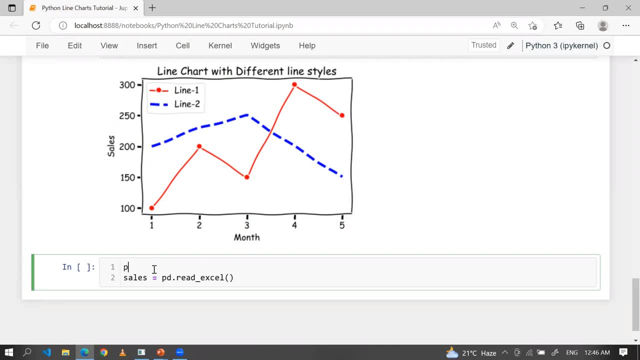 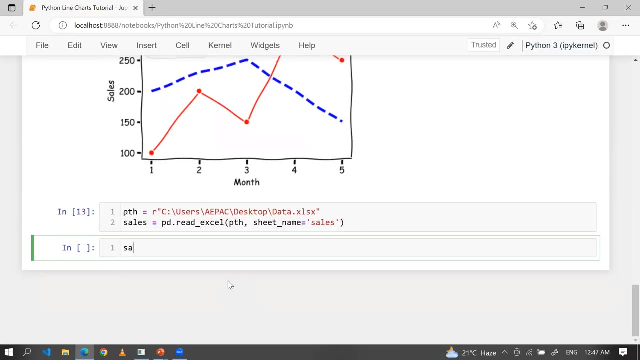 okay, and i am taking a variable, let's say pth. so this is the path guys i am taking. all right, and this particular path i am going to supply here and i am taking the sheet name, let's say sales guys. so now sales dot head. so this is the sales i have. okay, so i have generated the 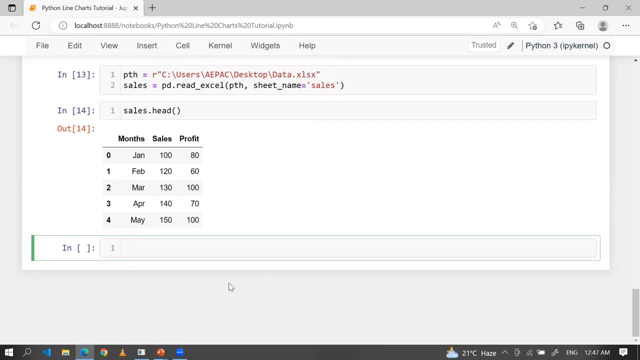 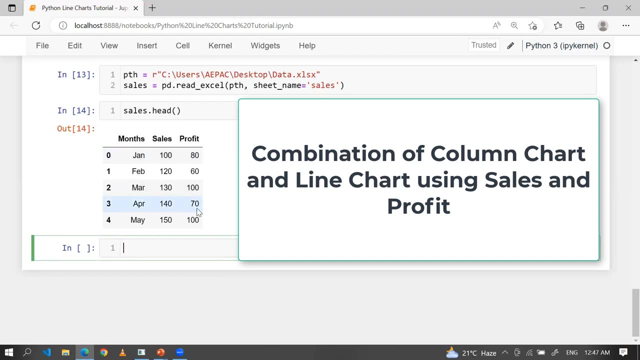 data month: wise, sales and profit. now i want to create the chart. so, guys, here, the sales, right, i want to represent as a column chart and the profit i want to represent as a line chart. okay, the combination of column and line chart i want to, you know, prepare. so what can i do here? let's say: 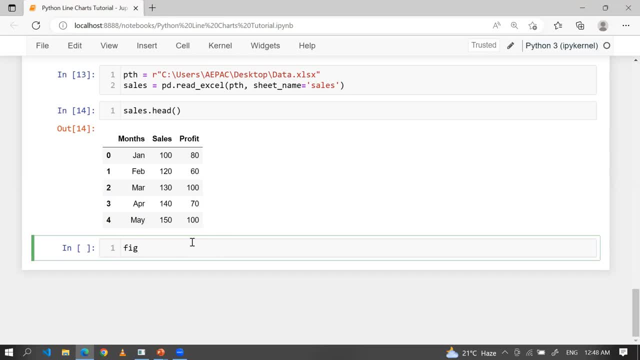 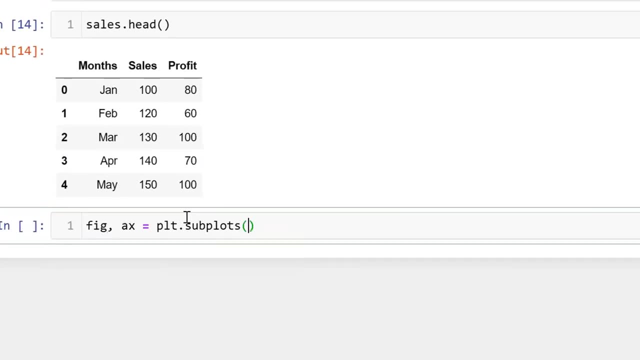 i am taking a simple. i can use here the fig and axis, okay, so equal to plt dot subplots got it. and here the fig size equal to, let's say, 10 by 3. okay, so you can customize in case you want to do it. so x is dot bar chart and guys, i am taking here the sales and you know months. similarly, i 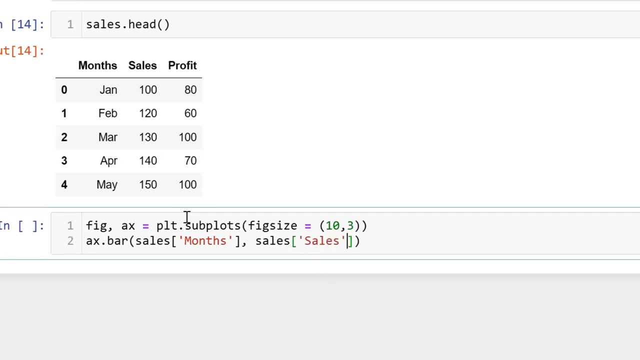 want the sales column simple and, guys, i want to supply the color equal to, let's say, dark blue, and you know what will be. the label of this particular chart is a sales. similarly, i want to plot the line chart so simple: sales. i want month and the sales i want to show. 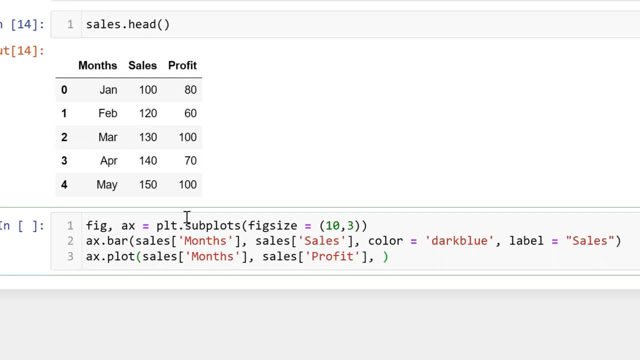 the profit. and again, you can supply the color, right. so let's say, color equal to you know, red color i want to supply, okay, and label equal to profit make sense. and now again, axis, which are set x label. and here, guys, this is the month and x is dot. set y label. 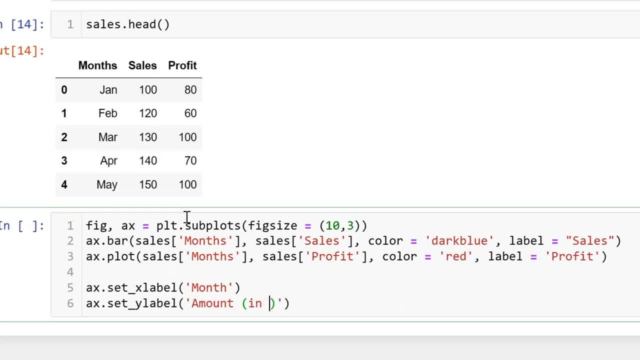 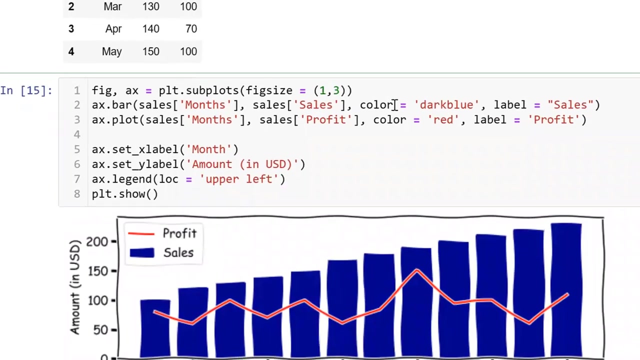 amount in in usd, got it. and then x dot legend: if you want to supply, let's say, lock equal to. now i want to upper left, whatever right and plt dot show. now let me run this. so guys look at this, okay. so let me you change the fig size. for an example, i want you know 12 and 4. okay, so now it is good to read. 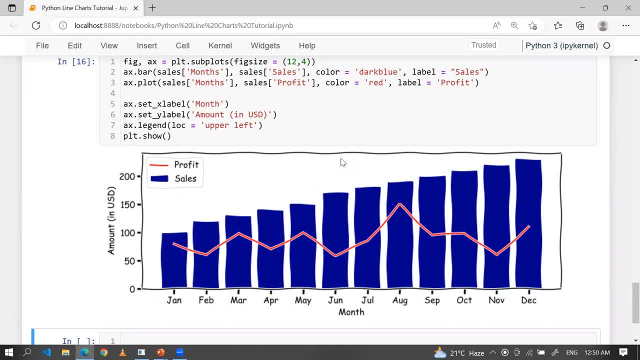 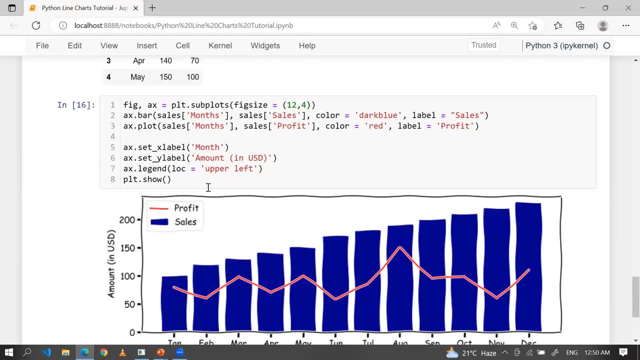 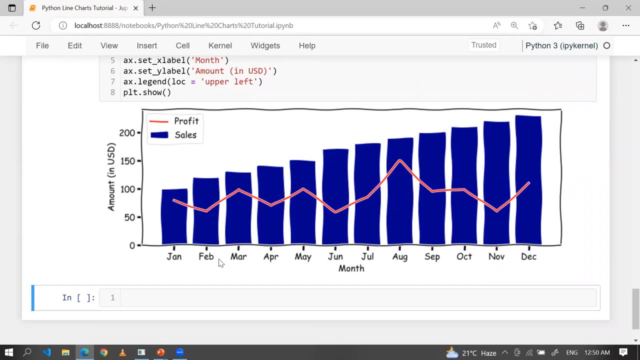 all right, so that's how you can create the chart. okay, so this is very easy to create. i hope you understood this chart. now let me show you the sales as a column chart and quantity and profit as a line chart, to see the difference. what i'm saying: sales should be a column chart and quantity. 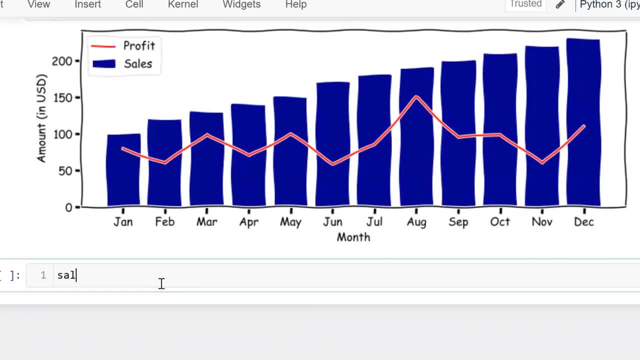 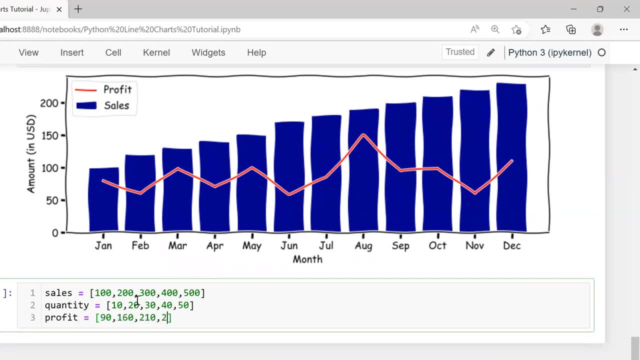 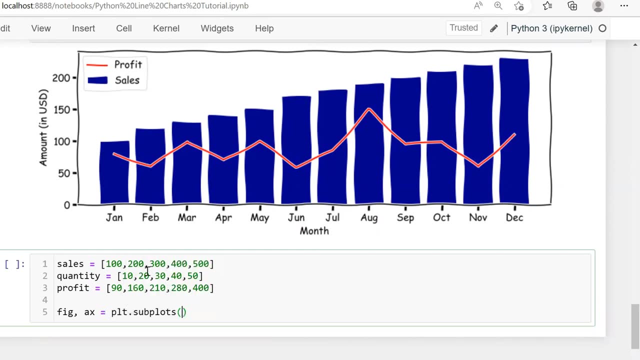 and profit i want to show as a line chart. so i am taking a sales as a random number. okay, any random information you can take. so here again, the same thing i am doing here which i did earlier and here axis, dot, bar graph guys. so np dot, arrange. some people call a range. 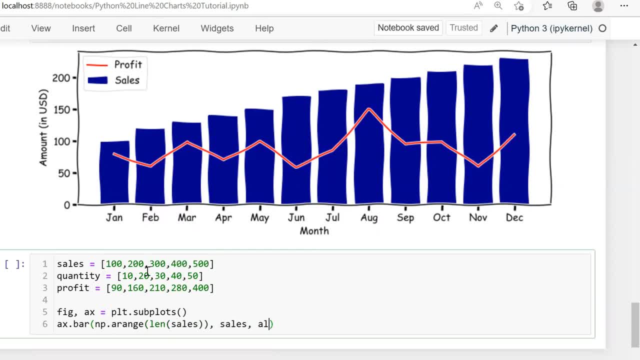 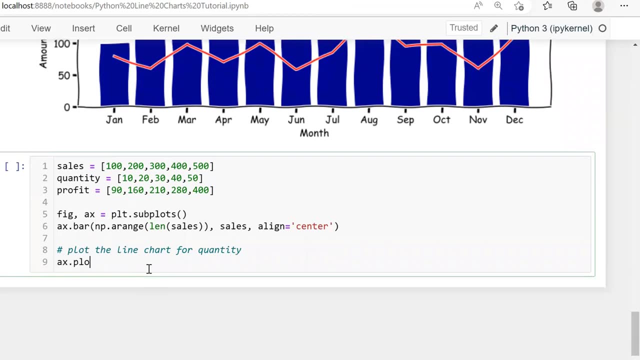 the length of sales. you know sales guys and i want to align into center, center, and here i'm going to plot the line chart for quantity. okay, so what can i do? access, dot, plot, np, dot, a range, and here length of quantity and simple quantity and color equal to red and line. 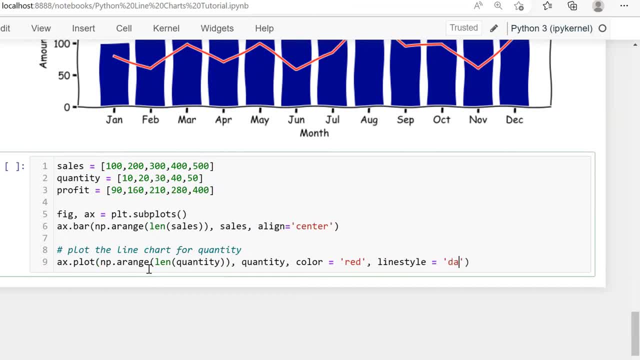 style equal to. guys dashed and again now plot the line chart for profit. again the same line. let me copy this. and here, guys, i want profit and the color should be- let's say it should be changed- orange and dotted, dotted line i want. and now adding labels and annotations. so what can i do here? 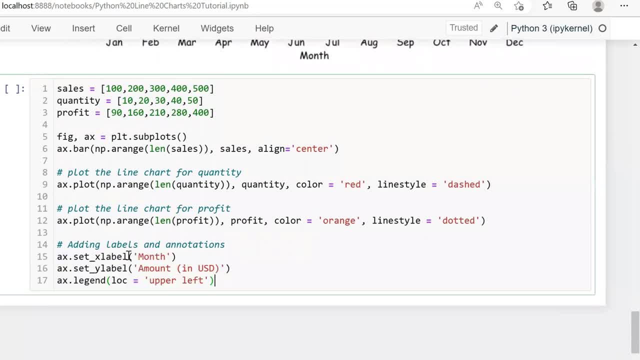 let me copy this paste here: set x label month. and, guys, one more thing i want to you know, set x sticks np, dot a range length of sale, it should be np. and here one more thing, guys. and here, guys, legend i am going to supply to it by this layerità tap on top of here. 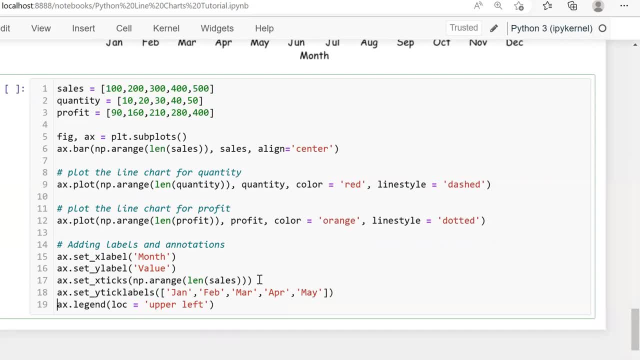 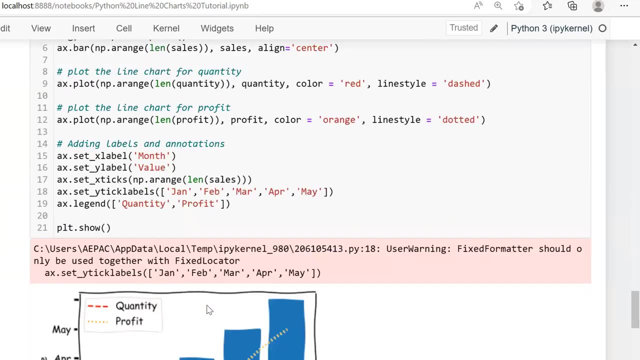 you know this is the sql i want to set up. going toெace feet us, the all these three shapes here, legend, i am going to supply and i am going to change the name of the legend. let's say i am going to supply, for an example, quantity and profit. all right guys. now pltshow, okay. 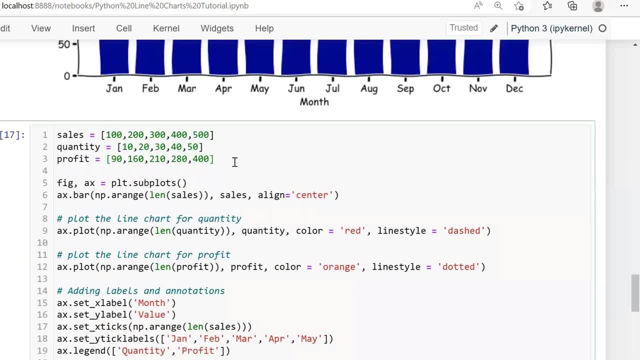 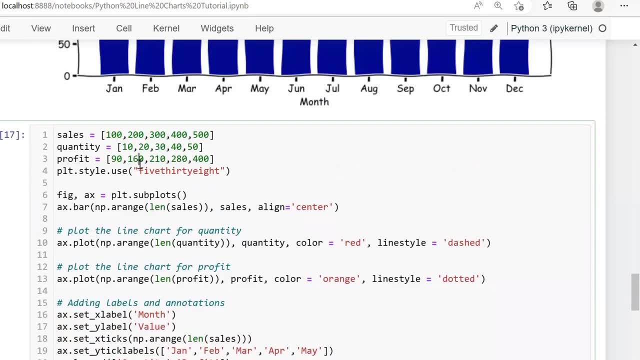 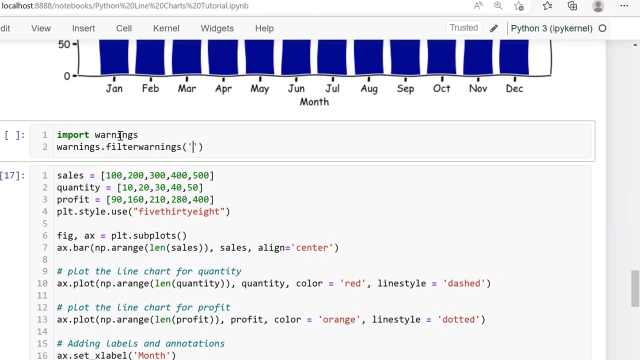 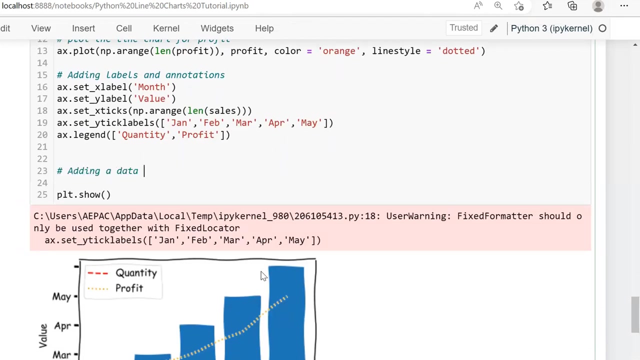 so look at this. and now let me do one thing here: plt, dot style, dot use here, guys, uh, one more thing. so let me import another library to remove this warning. so import warning warnings, dot filter warnings. and i want to ignore this. and, guys, i am doing one more thing: adding our data labels. 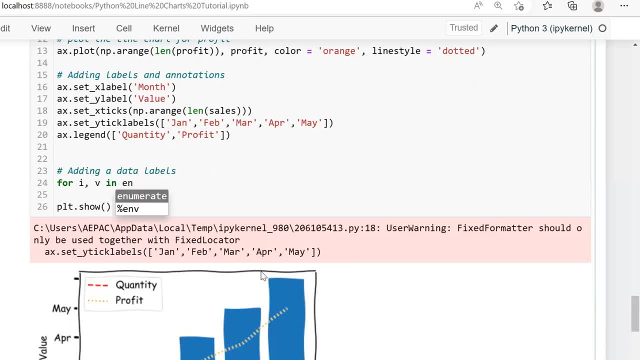 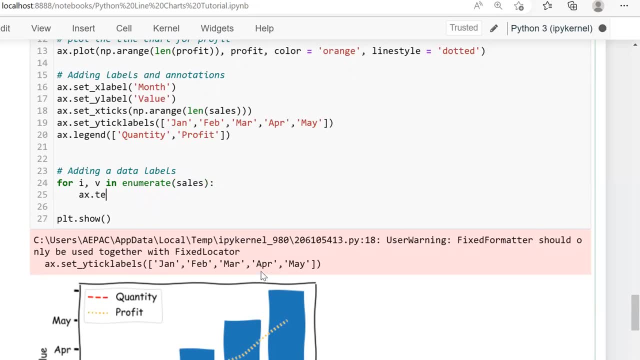 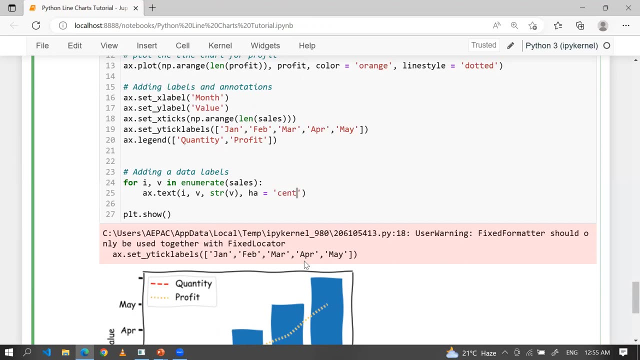 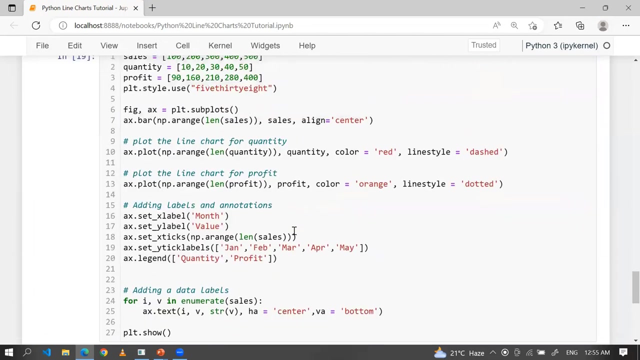 okay, again same thing. so in enumerators- and i am using here the sales and text and guys- same thing. and horizontal alignment is a center and vertical alignment equal to bottom, like this: okay, in case you want to change the fig size, so you can do the fig size with, let's say, 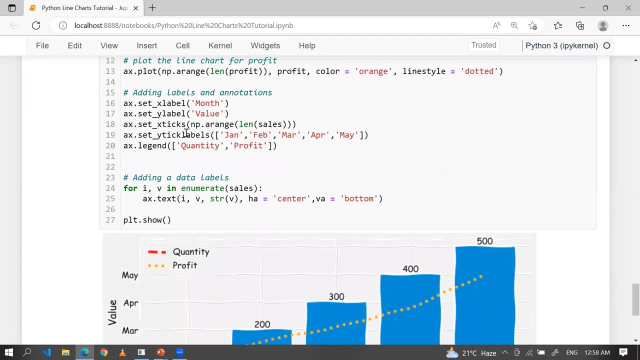 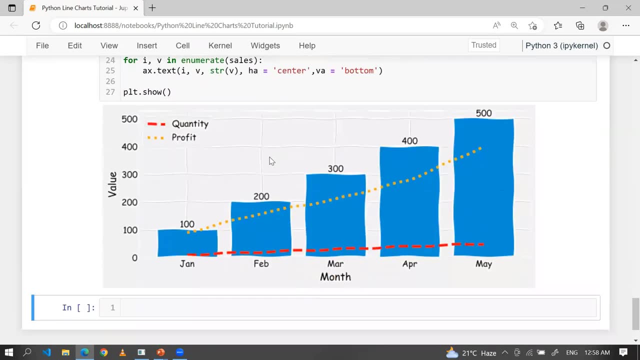 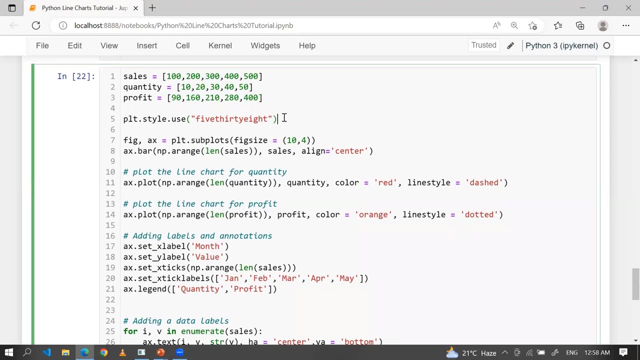 10 by 4.. so, guys, uh, here we are doing some mistakes, so this has to be on x-axis, right? so now let me run this. okay, now it is perfect, okay. so again, it is a very easy: create the sales quantity and profit, and I am using this style from the matplotlib and this: 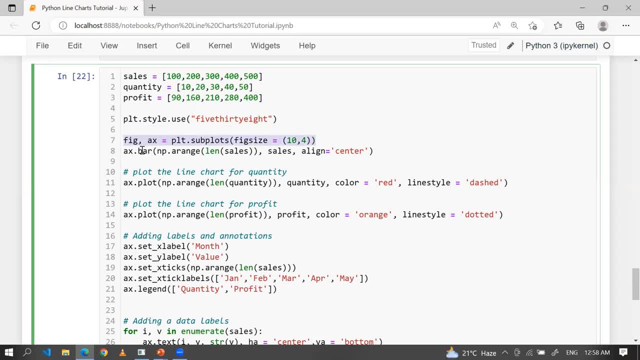 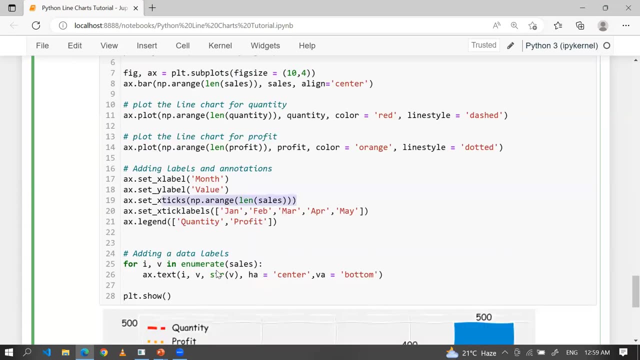 is the- you know- figure, size and axis. and on the axis, let's say, using the axis, I am going to create the bar chart and then I am going to create a plot chart based on quantity and profit, and this labels for x axis and this is the y axis and this is the x ticks. okay, these are the sales, all right. 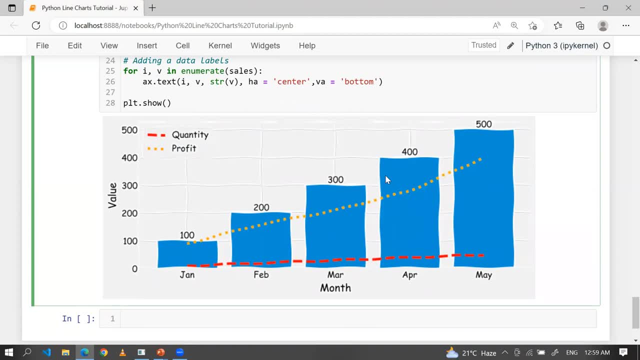 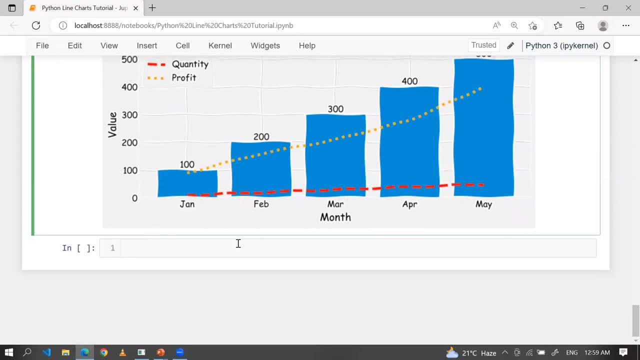 and here I am going to: you know supply, you know some data labels, so this is very easy to do that. and guys, sometimes, let's say, people are saying can you create a target versus sales? so how you can plot target versus say, let's say you are going to set the target for an example, 1000. 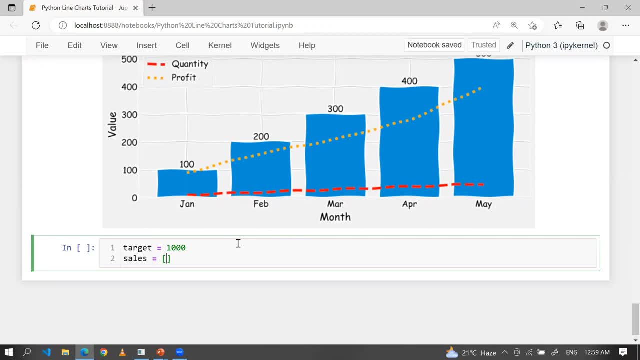 and again this target: you are doing some sales, all right, so like this. after that, let's say: you are doing some sales, all right, so like this. after that, let's say: you are doing some, let's say you want to show so this particular sales. so what I am doing here, this is my target. 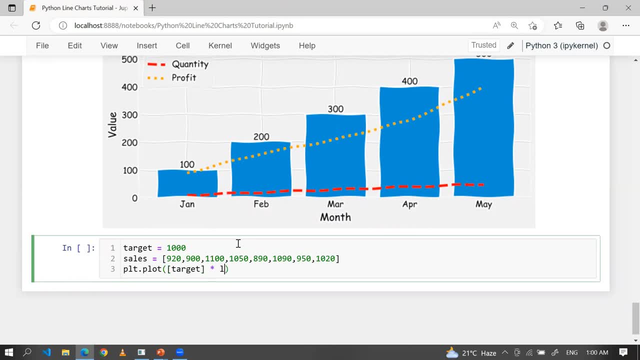 okay, so entire list I am taking. multiply by whatever the length of sales. okay, so 1000. I am repeating multiple times now: label equal to, let's say, target, and here plt dot plot, so let's sales. and label equal to. you want to show this label: plt dot legend. we want to show plt dot x. 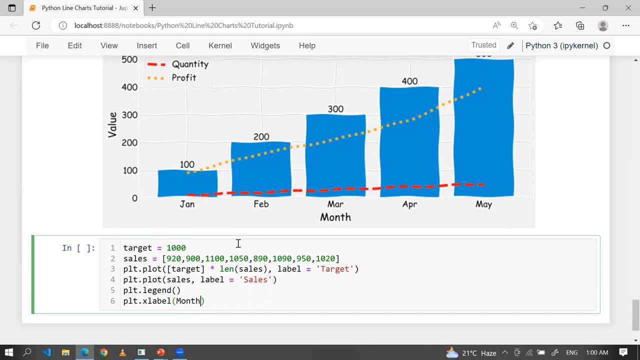 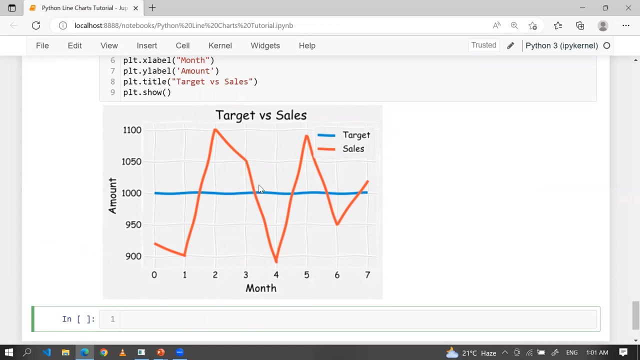 label, let's say month, right, and plt dot y label equal to, and here plt dot title I want to supply. let's say target versus sales: okay, and that chart I want to show. this is my particular target and against this target I am achieving this sales okay, so that's how you can do that. let me give. 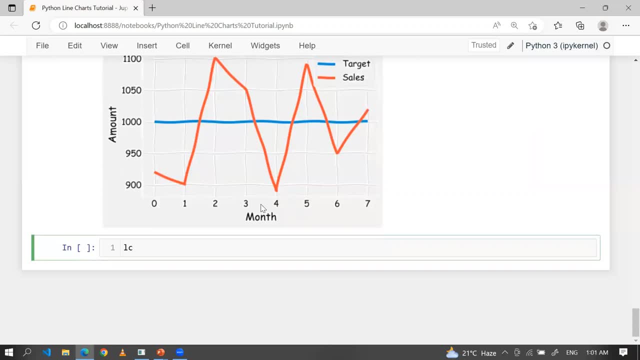 you a couple of examples of how you can do that. let me give you a couple of examples of how you can do that. let me give you a couple of examples of how you can do that. let me give you a couple of more examples on live data. so what I am doing here, so I'm, I am reading the data from again. more examples on live data. so what I am doing here. so I am, I am reading the data from again. more examples on live data. so what I am doing here. so I am, I am reading the data from again. from that Excel, so from the path. from that Excel, so from the path. 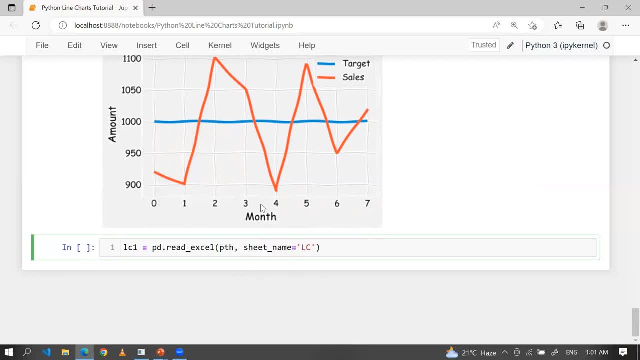 from that Excel, so from the path, and here the sheet name. I am using line and here the sheet name. I am using line and here the sheet name. I am using line number one. all right, so this is LC one number one. all right, so this is LC one. 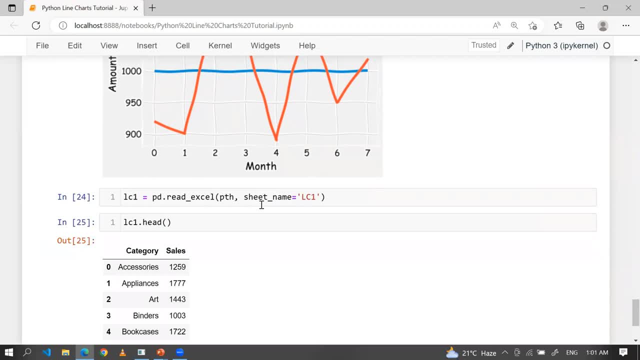 number one. all right, so this is LC one dot had now. I want to show you the chart dot had. now. I want to show you the chart dot had. now I want to show you the chart. you know sales by category. I want to. so you know sales by category, I want to. so 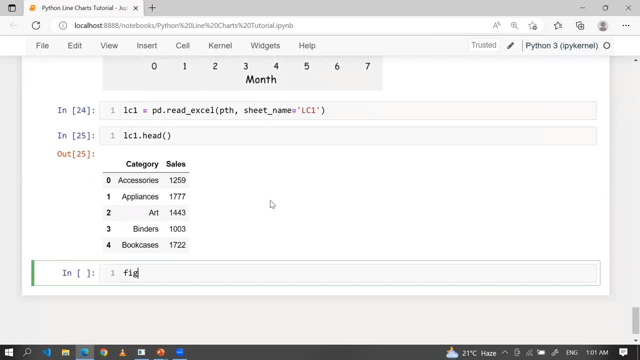 you know, sales by category. I want to, so okay. so sales by category: miss again, I okay. so sales by category: miss again, I okay. so sales by category: miss again. I am taking a fig and access equal to PLT. am taking a fig and access equal to PLT. 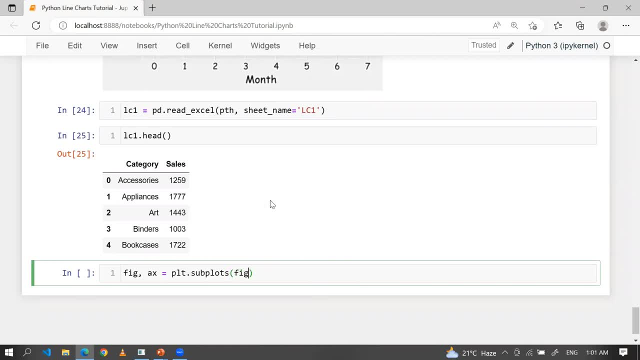 am taking a fig and access equal to PLT, dot subplots. and here I am going to dot subplots, and here I am going to dot subplots, and here I am going to assign the fig size. let's say 10 by 4. assign the fig size, let's say 10 by 4. 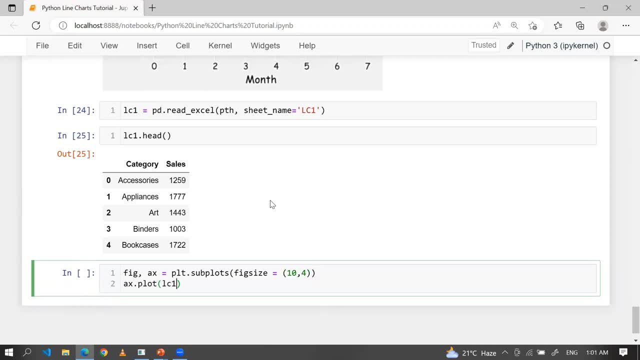 assign the fig size, let's say 10 by 4, and here X is dot plot LC one. and let's, and here X is dot plot LC one. and let's, and here X is dot plot LC one. and let's say, guys, I am taking a category on the. 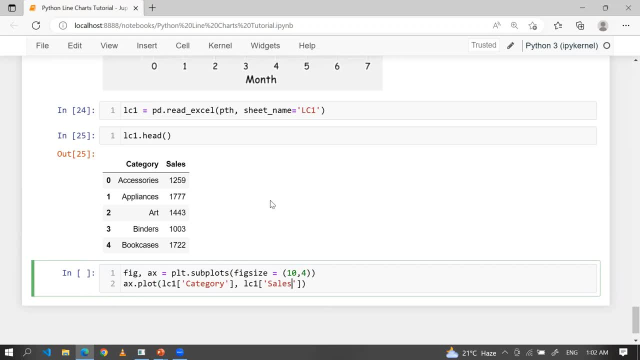 say, guys, I am taking a category on the. say, guys, I am taking a category on the y-axis LC one. let's say I am taking a y-axis LC one. let's say I am taking a y-axis LC one. let's say I am taking a sales. and now, guys, I am going to set the. 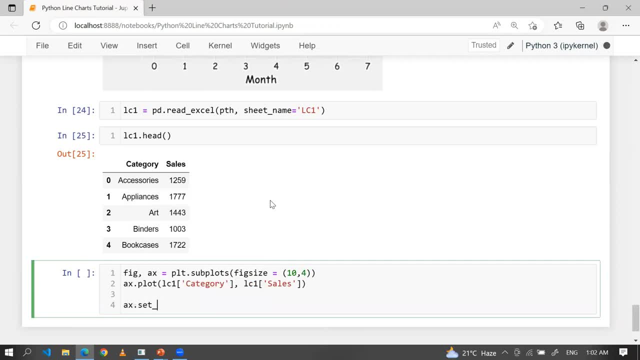 sales. and now, guys, I am going to set the sales. and now, guys, I am going to set the chart title and axis label. so what can I? chart title and axis label. so what can I? chart title and axis label. so what can I do here? do here? 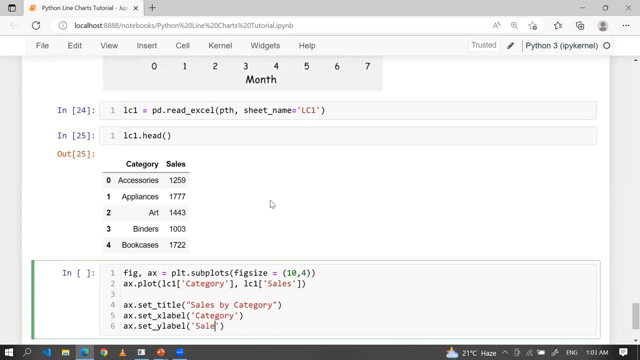 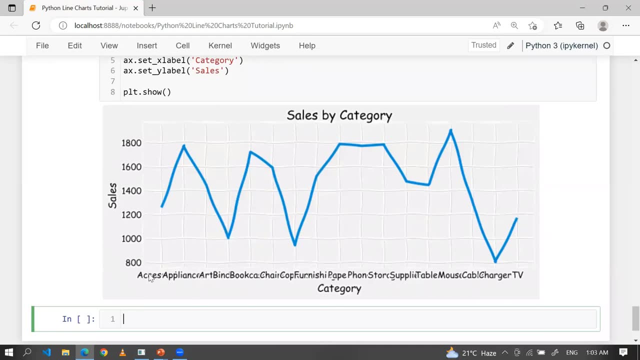 do here directly. I'm using here PLT dot show directly. I'm using here PLT dot show directly. I'm using here PLT dot show. so look at this. all right. so, guys, now you so look at this. all right. so, guys, now you so look at this. all right. so, guys, now you can see here these categories, right. 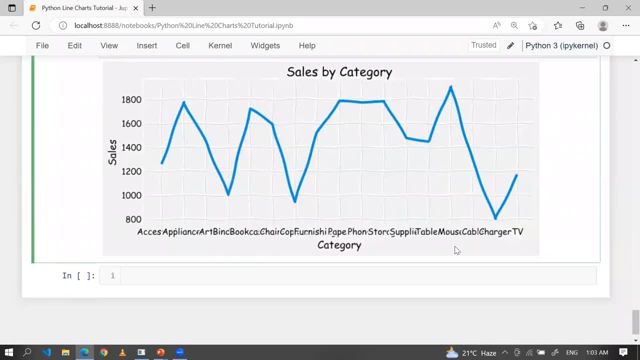 can see here these categories, right. can see here these categories, right. it is not in readable mode, so what can I? it is not in readable mode, so what can I? it is not in readable mode, so what can I do? so this is the part of X, X's. so what? 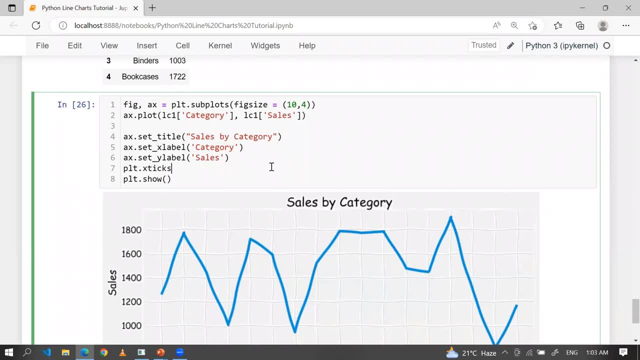 do so? this is the part of X- X's. so what do so? this is the part of X- X's. so what can I do here? PLT dot X ticks and I am. can I do here? PLT dot X ticks and I am. can I do here? PLT dot X ticks, and I am going to use the rotation rotation. 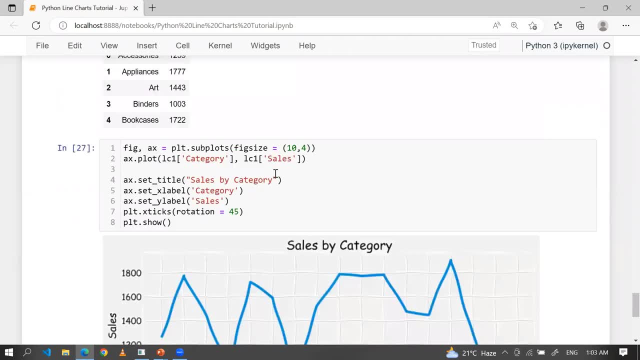 going to use the rotation rotation. going to use the rotation rotation equal to, let's say, 45 degree or 90. equal to, let's say, 45 degree or 90. equal to, let's say, 45 degree or 90 degree. you can use whatever right now. 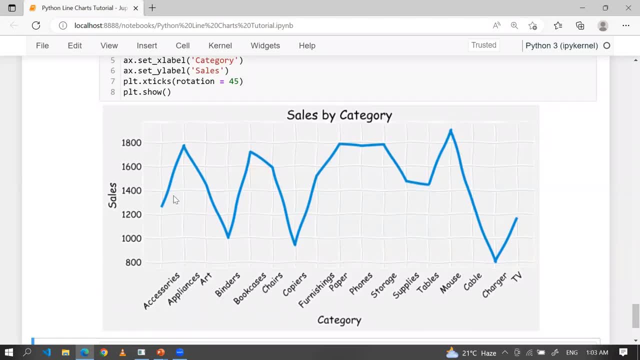 degree: you can use whatever right now. degree: you can use whatever right now. you, everybody can read these. you know you, everybody can read these. you know you, everybody can read these. you know category, and these are the saves alright category, and these are the saves alright category and these are the saves alright. and now, for an example, if you want to, 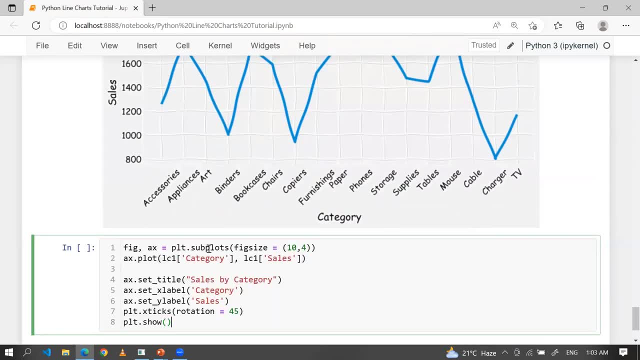 and now for an example, if you want to. and now for an example, if you want to. you know some supply, you know some. you know some supply, you know some, you know some supply. you know some colors and some style so you can use colors and some style so you can use. 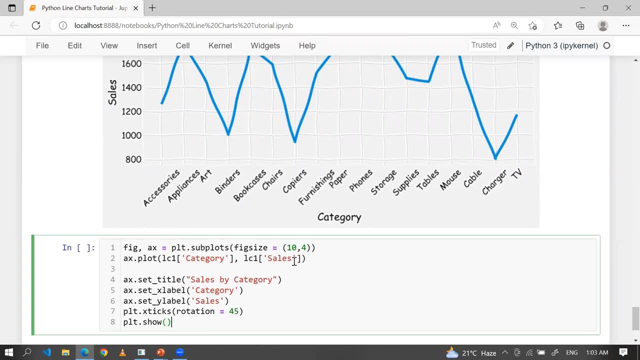 colors and some style so you can use this particular part easily. so I am this particular part easily, so I am this particular part easily. so I am telling you, let's say I want you know. telling you, let's say I want you know. telling you, let's say I want you know, color equal to blue and the marker I. 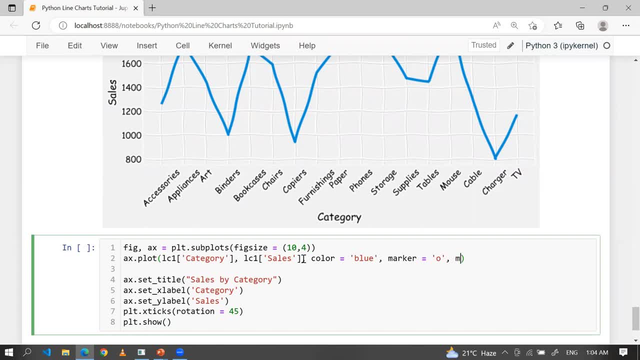 color equal to blue and the marker I color equal to blue and the marker I want. let's say oh and you want to want, let's say oh and you want to want, let's say oh and you want to sales right. so, and here I want legend as. 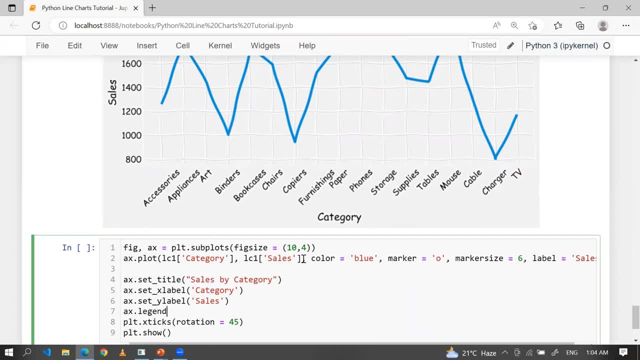 sales, right so, and here I want legend as sales, right so? and here I want legend as well. so, axis equal to legend and simple. well, so, axis equal to legend and simple. well, so, axis equal to legend and simple. I can show you, okay. so that's how you. 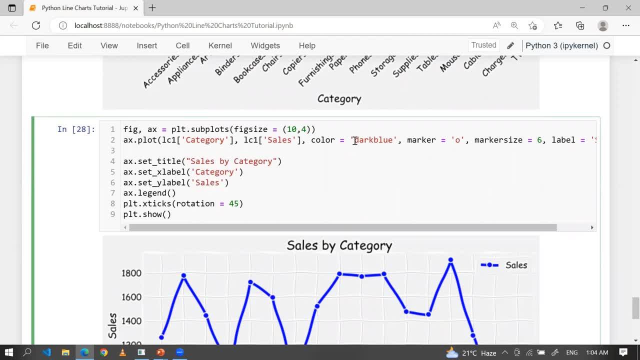 I can show you okay. so that's how you. I can show you okay. so that's how you can do that. let's say: I want dark blue. can do that. let's say: I want dark blue can do that. let's say: I want dark blue. look at this. so now everybody can read. 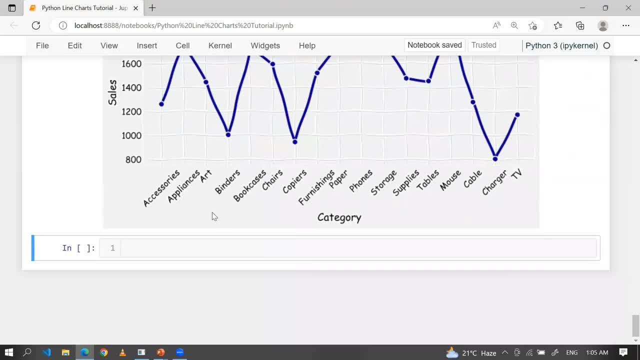 look at this, so now everybody can read. look at this, so now everybody can read: this, got it. and now, guys I want to this, got it. and now, guys I want to this, got it. and now, guys, I want to create a multiple line chart. okay so, create a multiple line chart, okay so. 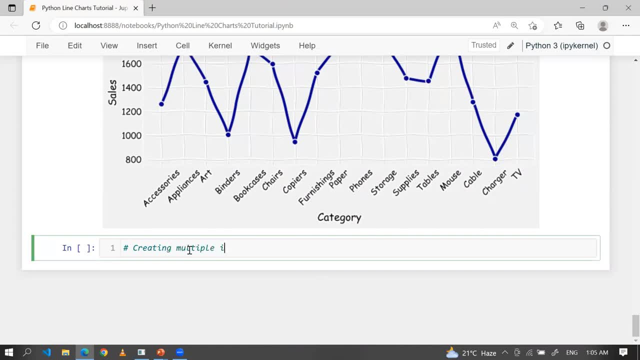 create a multiple line chart. okay, so what I'm doing here, creating multiple. what I'm doing here, creating multiple. what I'm doing here, creating multiple line chart. so what can I do here? let's line chart. so what can I do here? let's line chart. so what can I do here? let's say LC to equal to. again, I am reading: 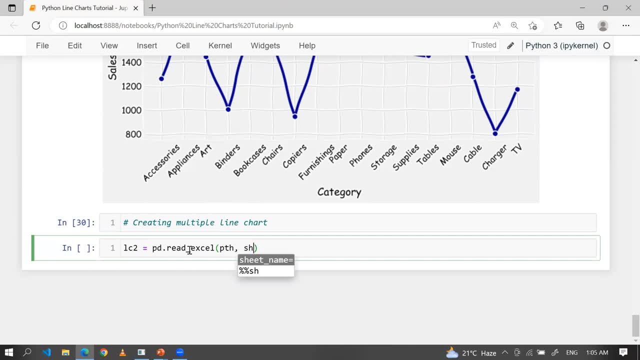 say LC to equal to again I am reading: say LC to equal to again. I am reading the data from the Excel and from the. the data from the Excel and from the. the data from the Excel and from the path and the sheet name: equal to. let's. 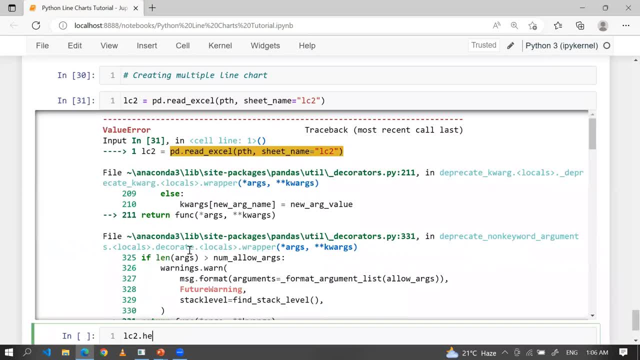 path and the sheet name equal to let's path and the sheet name equal to, let's say, LC to. so now, LC to dot head- okay, I say LC to. so now LC to dot head- okay, I say LC to. so now LC to dot head, okay. I think is the case sensitive. so look at. 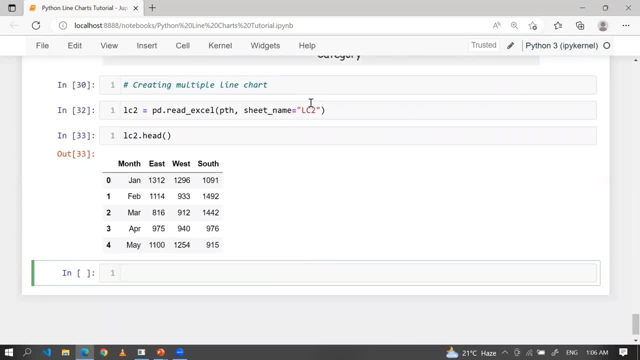 think is the case sensitive. so look at think is the case sensitive. so look at this. so right now I have a month and I this. so right now I have a month and I this. so right now I have a month and I have a reason why sales okay. so I want. 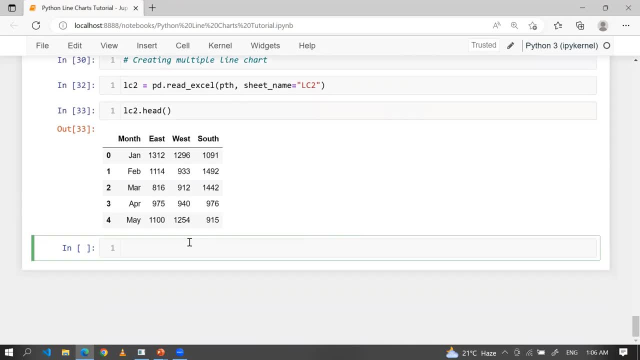 have a reason why sales okay, so I want have a reason why sales okay, so I want to you know. see the difference based on to you know. see the difference based on to you know. see the difference based on my reason. so what can I do? here I am. 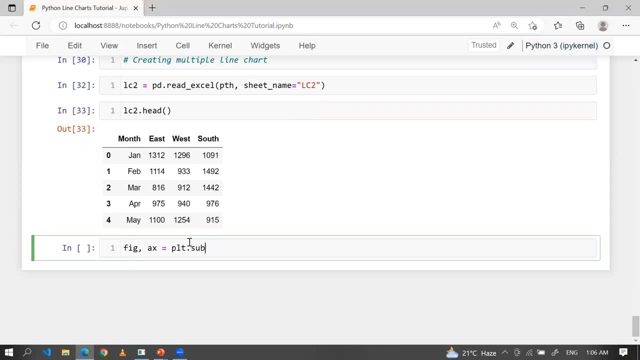 my reason. so what can I do here? I am my reason, so what can I do here? I am going to create a same thing. so PLT dot going to create a same thing. so PLT dot going to create a same thing. so PLT dot subplots, and here big size equal to. 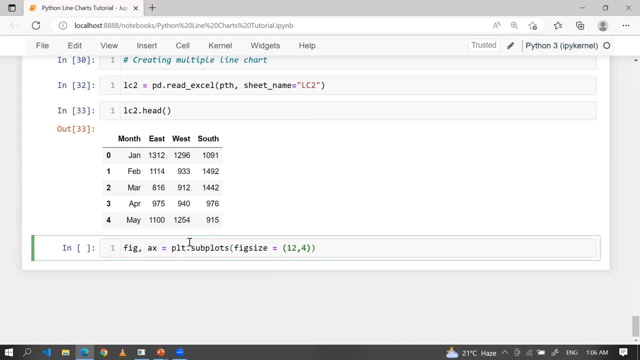 subplots, and here, big size equal to subplots, and here, big size equal to. let's say, guys, you know 12 by 4. let's say, guys, you know 12 by 4. let's say, guys, you know 12 by 4, LC to and I am taking a month and LC to. 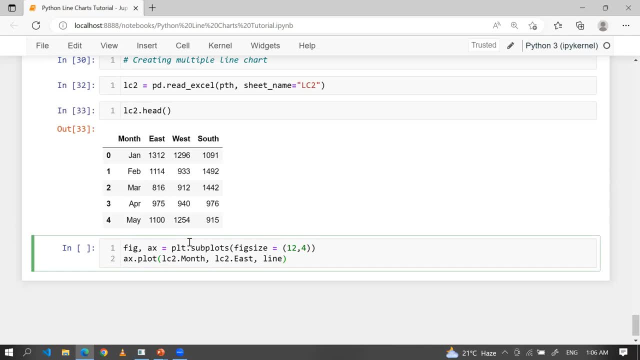 LC to, and I am taking a month and LC to, LC to, and I am taking a month and LC to again I am taking East and the line. again I am taking East and the line. again I am taking East and the line width, guys, I am taking two and the color. 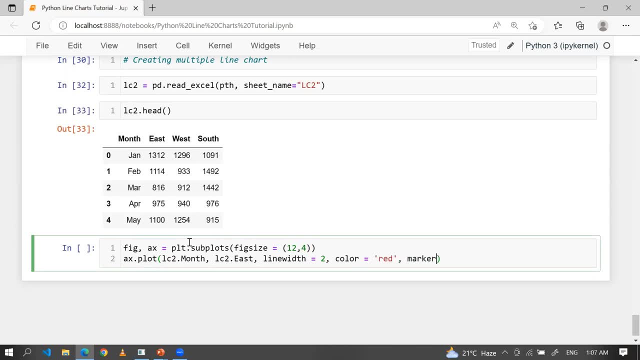 width guys, I am taking two. and the color width guys- I am taking two. and the color equal to red and the marker which is oh, equal to red. and the marker which is oh, equal to red. and the marker which is oh. you want to supply the marker size right? 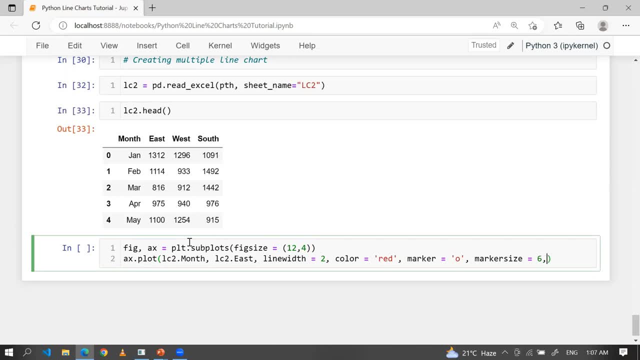 you want to supply the marker size right. you want to supply the marker size right. marker size equal to six and the label marker size equal to six and the label marker size equal to six and the label equal to, let's say, East right, equal to, let's say East right. 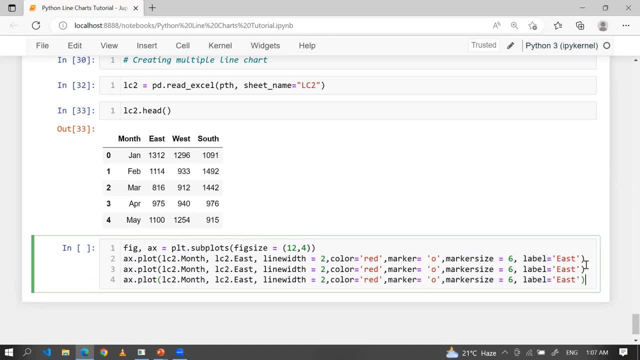 equal to, let's say, East right and similarly, what can I do? and let me, and similarly, what can I do and let me, and similarly, what can I do? and let me paste this: so this is for West, this is. paste this. so this is for West, this is. 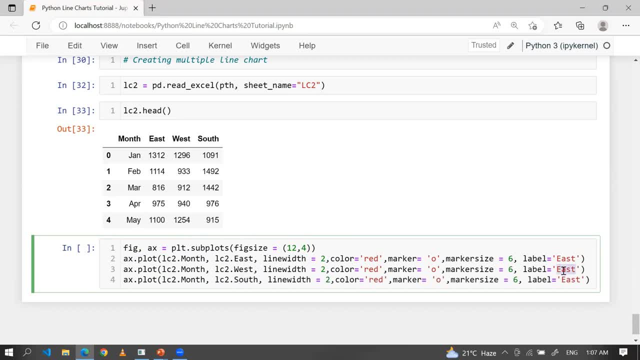 paste this. so this is for West, this is for South, and this is also West and South for South, and this is also West and South for South, and this is also West and South. let me change the color as well. let me change the color as well. let me change the color as well. let's say green and blue. and, guys, you can. 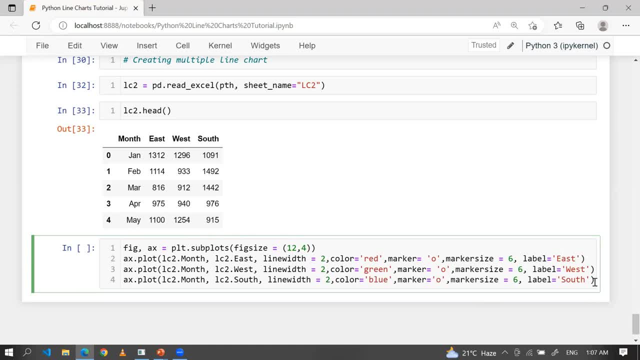 let's say green and blue, and guys you can. let's say green and blue, and guys you can supply the. you know the hexadecimal supply, the. you know the hexadecimal supply, the. you know the hexadecimal color as well. okay, which I shown you in color as well. okay, which I shown you in. 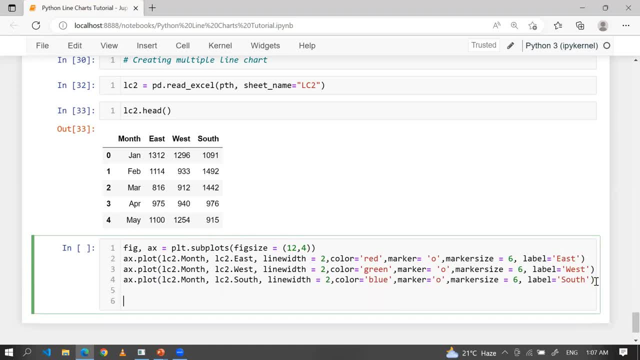 color as well, okay, which I shown you in the last session, and now I am going to the last session, and now I am going to the last session, and now I am going to set that title, so X is dot set title on. set that title, so X is dot set title on. 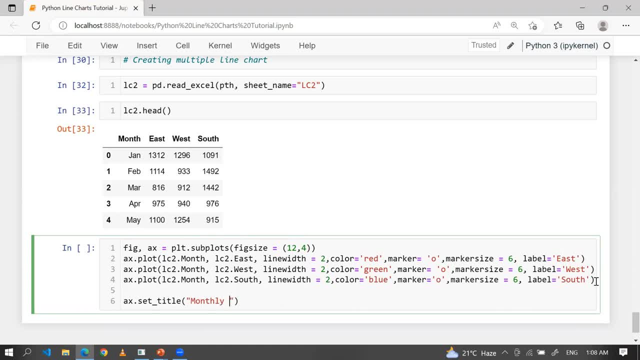 set that title. so X is dot set title on here month Lee sales by reason. and now here month Lee sales by reason. and now here month Lee sales by reason. and now axis dot set X label on the x-axis I am. axis dot set X label on the x-axis I am. 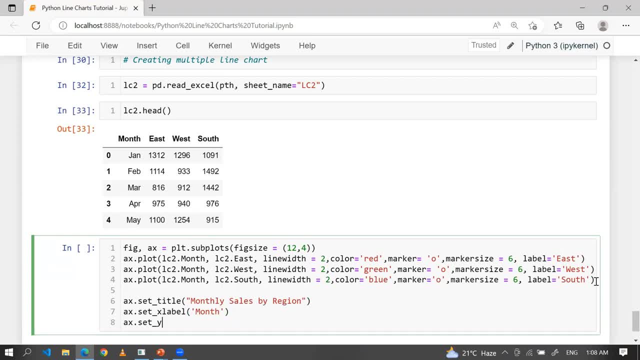 axis: dot set X label. on the x-axis: I am going to show you the month and X is going to show you the month and X is going to show you the month and X is dot set Y label. I am going to show you the dot set Y label. I am going to show you the. 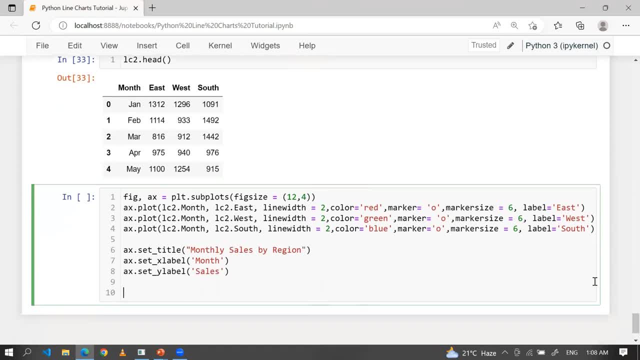 dot set Y label. I am going to show you the sales and again I have to roll dot set Y label. I am going to show you the sales and again I have to roll dot set Y label. I am going to show you the sales and again I have to roll it. my x-ticks, sorry, and the. 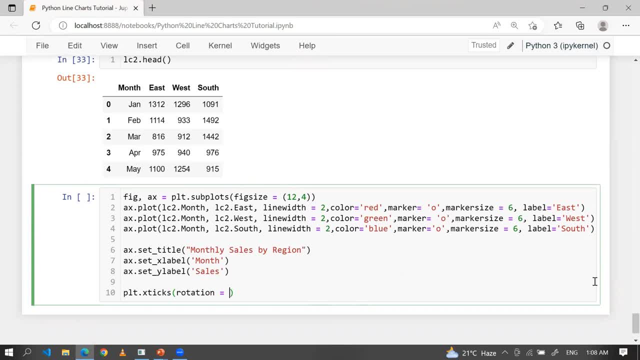 it my x-ticks sorry, and the it my x-ticks sorry. and the rotation equal to 45 degree and axis dot legend rotation equal to 45 degree and axis dot legend rotation equal to 45 degree and axis dot legend for an example lock equal to- let's. 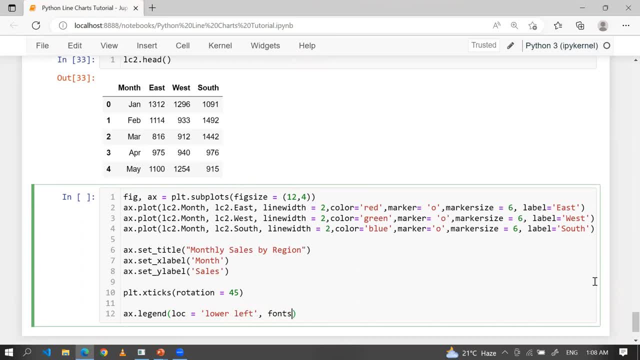 for an example lock equal to let's. for an example lock equal to, let's say, lower left. you want to change the size, say lower left. you want to change the size- say lower left. you want to change the size right. font size equal to 10 and PLT. 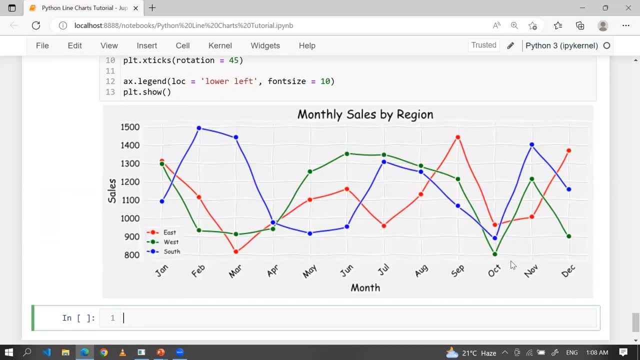 right font size equal to 10 and PLT right font size equal to 10 and PLT dot show: all right, so let me do here the dot show, all right. so let me do here the dot show, all right, so let me do here the 10. so, guys, using this multiple line of, 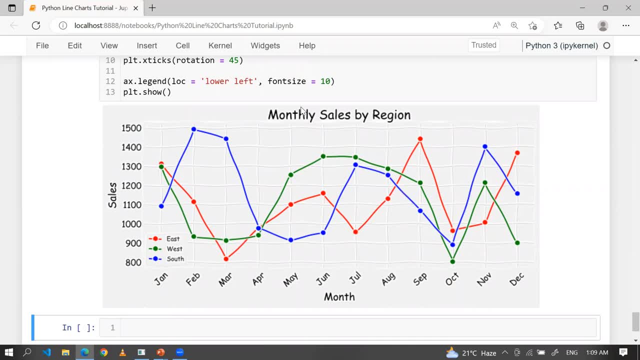 10. so, guys, using this multiple line of 10, so, guys, using this multiple line of chart, we can see the difference based on chart. we can see the difference based on chart. we can see the difference based on East, West and South against the month: East West and South against the month. 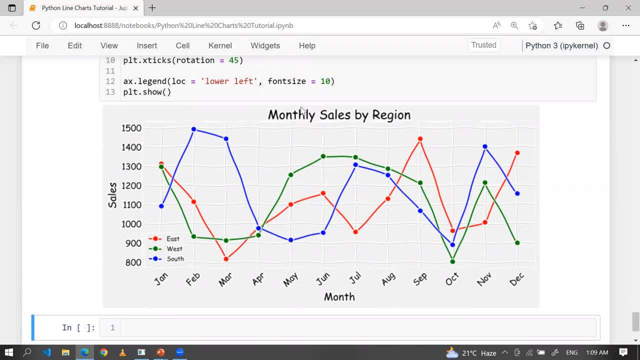 East, West and South, against the month. okay, so it is very easy to understand. okay, so it is very easy to understand. okay, so it is very easy to understand this particular part, all right. and guys this particular part, all right. and guys this particular part, all right. and guys in the last, I am going to show you how. 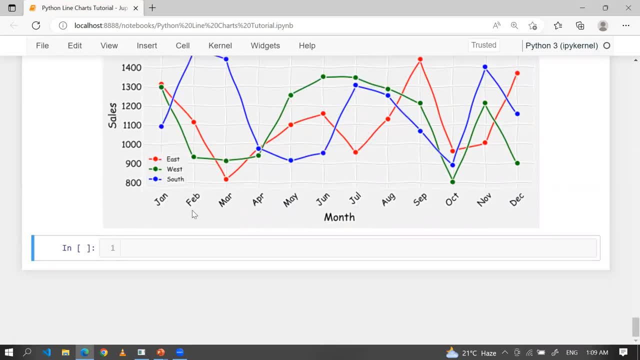 in the last, I am going to show you how. in the last, I am going to show you how you can create the chart another. you can create the chart another. you can create the chart another. different data set. so look at this. so different data set. so look at this, so. 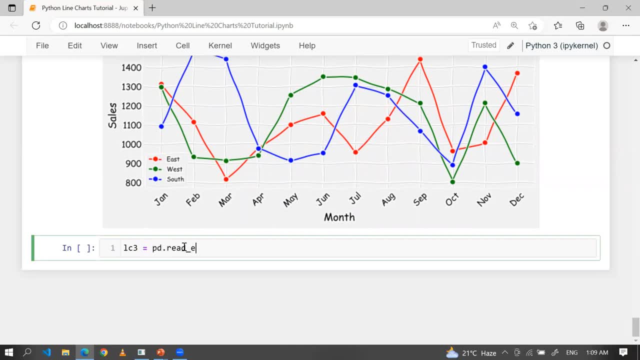 different data set. so look at this. so again: LC 3 equal to PD. dot read Excel again. LC 3 equal to PD. dot read Excel. again LC 3 equal to PD. dot read Excel again. I am reading my data from the sheet. again I am reading my data from the sheet. 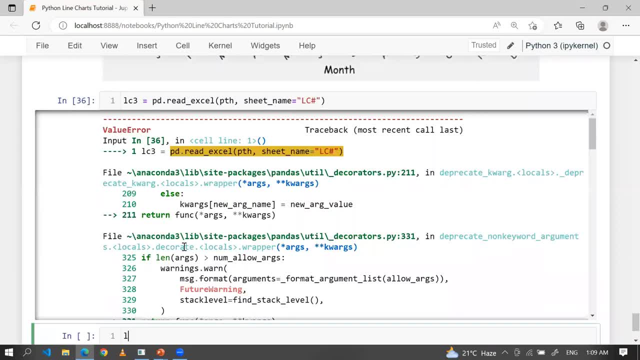 again. I am reading my data from the sheet: name: equal to LC 3, so LC 3, not hash. name: equal to LC 3, so LC 3, not hash name. equal to LC 3, so LC 3, not hash. so now let me show you this one. okay, so. 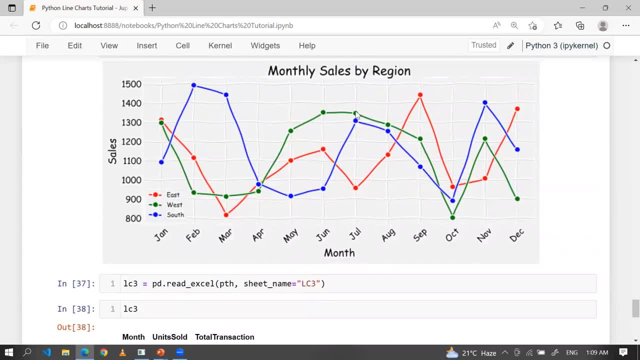 so now let me show you this one, okay, so. so now let me show you this one, okay. so see what I want for an example. let's say: see what I want for an example. let's say: see what I want for an example. let's say: I have created this line chart, I want. 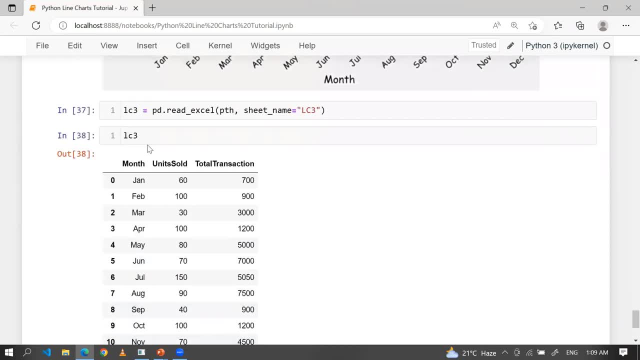 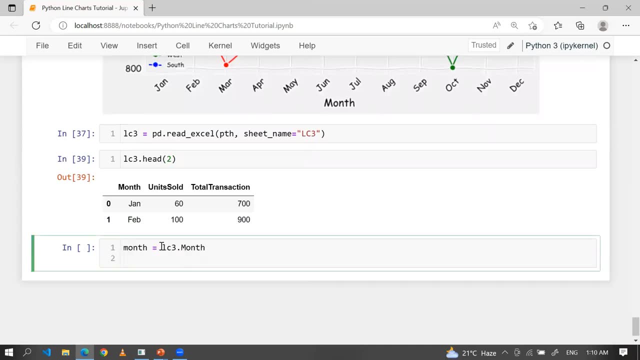 I have created this line chart. I want. I have created this line chart. I want the data label is as well on this chart. the data label is as well on this chart. the data label is as well on this chart: month and, for an example, unit sold. let's. 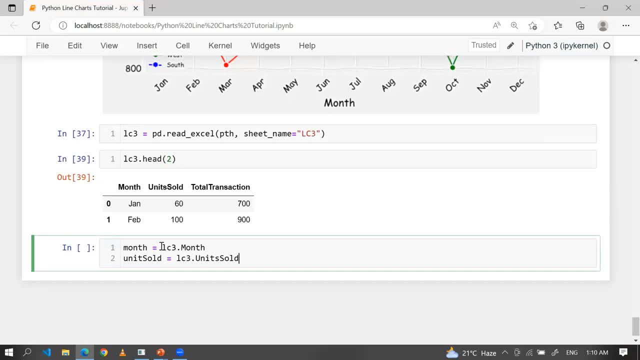 month and for an example unit sold, let's month and for an example unit sold. let's say LC 3 and unit sold and total. say LC 3 and unit sold and total. say LC 3 and unit sold and total transaction total equal to LC 3 total. 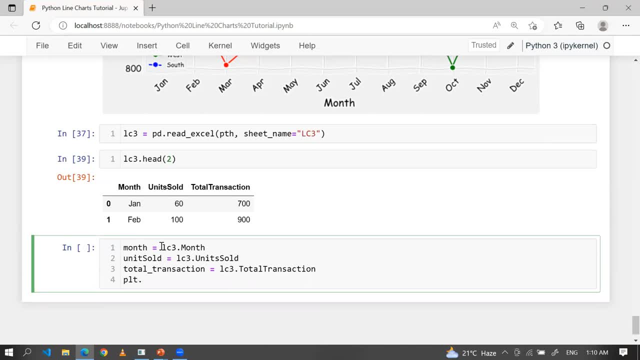 transaction total equal to LC 3 total transaction total equal to LC 3 total transaction. all right, I am using here transaction. all right, I am using here transaction. all right, I am using here again that use, let's say see bond, and again that use, let's say see bond, and. 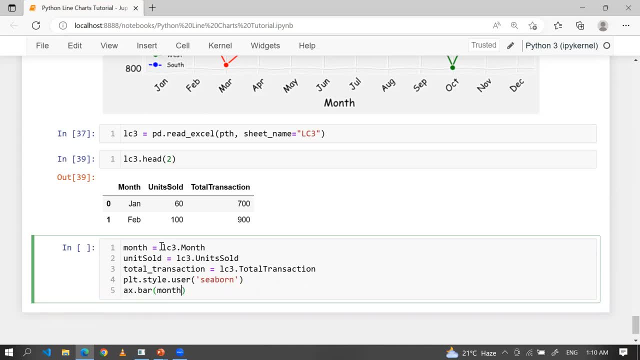 again that use. let's say, see bond. and here now I'm going to create the chart. here now I'm going to create the chart. here now I'm going to create the chart: dark blue. I'm going to change the style: dark blue, I'm going to change the style. 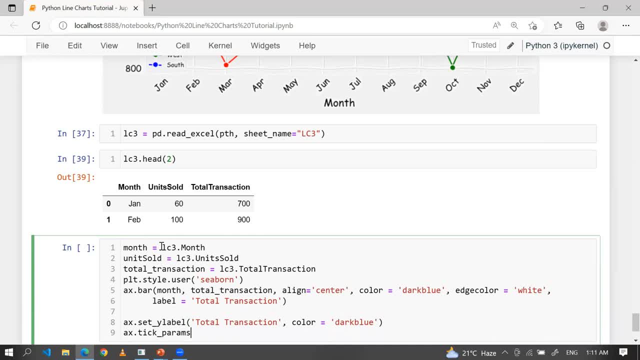 dark blue. I'm going to change the style in this chart and X params and axis in this chart and X params and axis in this chart and X params and axis equal to Y and the label color equal to. equal to Y and the label color equal to. 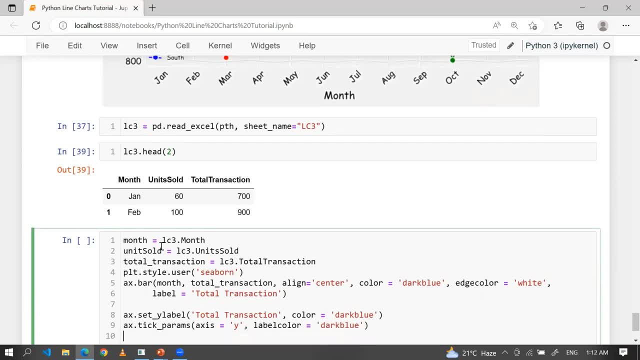 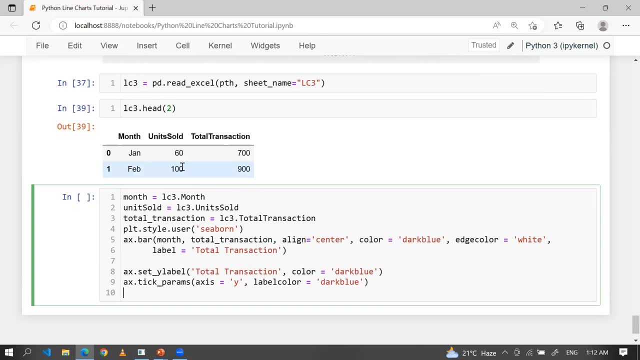 equal to Y and the label color equal to dark blue. dark blue, dark blue. all right again. this. all right again this. all right again. this transaction, again this transaction. I want to transaction again this transaction. I want to transaction again this transaction. I want to show this unit sold as a line chart. 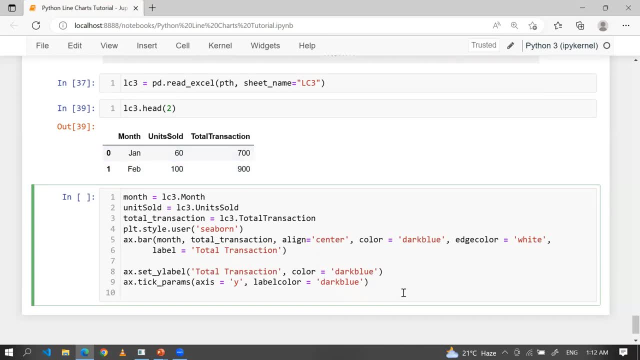 show this unit sold as a line chart. show this unit sold as a line chart. okay, so I am going to change the axis. so okay, so, I am going to change the axis. so okay, so, I am going to change the axis. so how can I change the axis? so, guys, what? 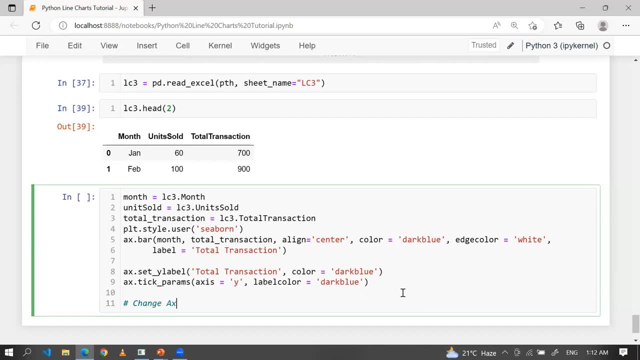 how can I change the axis? so, guys, what? how can I change the axis? so, guys, what I am doing here: change axis okay. so second, I am doing here: change axis okay. so second I am doing here: change axis. okay. so second set of y-axis with new axis I am. 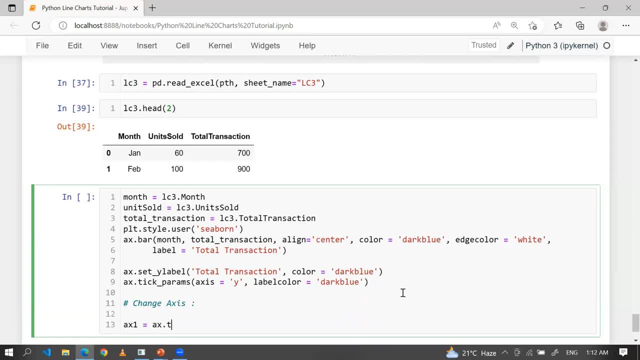 set of y- axis with new axis. I am set of y- axis with new axis. I am going to do here: X is 1 equal to X is dot going to do here. X is dot going to do here. X is dot, twin X. okay, so what do you mean by this? let 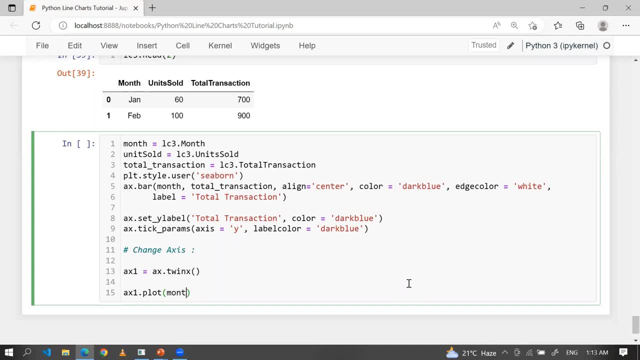 twin X, okay. so what do you mean by this? let twin X, okay. so what do you mean by this? let me tell you X is 1 dot plot month. me. tell you X is 1 dot plot month. me. tell you X is 1 dot plot month. unit sold. color equal to red line width. 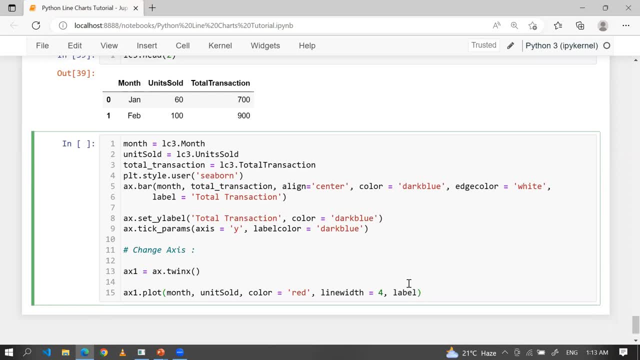 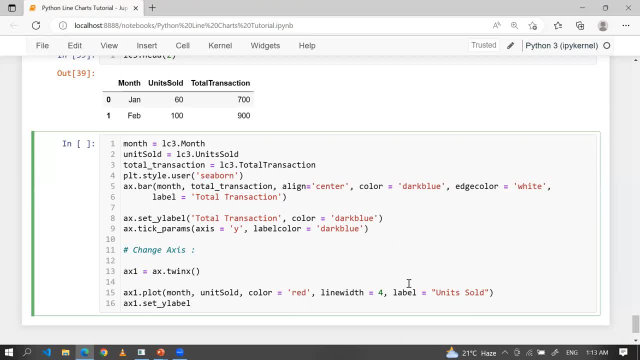 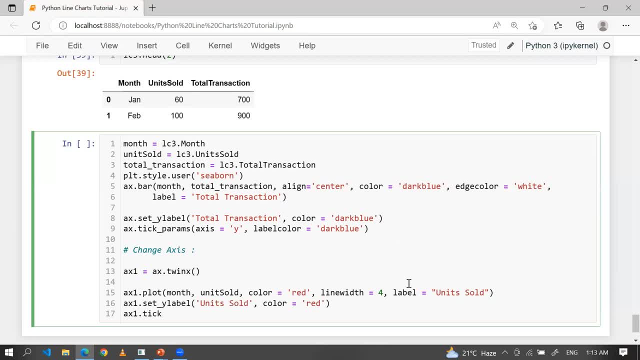 supply any color the same color- red supply any color the same color- red color I want, and X is 1 dot tick color I want and X is 1 dot tick color I want and X is 1 dot tick params, and here, that is, X is equal to. 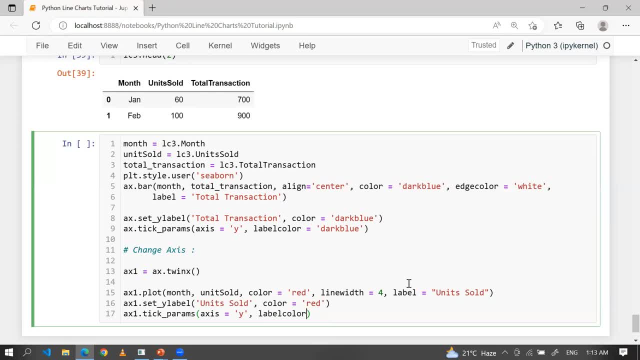 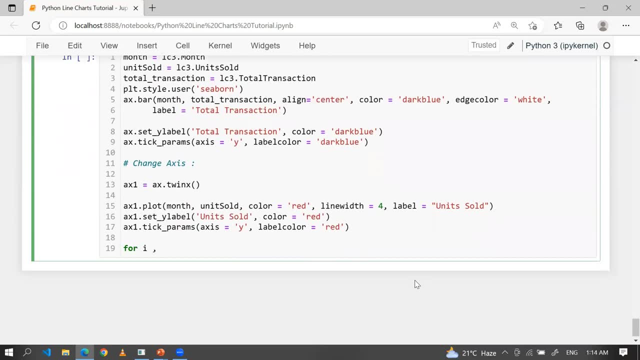 params, and here that is X is equal to params, and here that is X is equal to Y, and label color equal to again say red Y, and label color equal to again say red Y, and label color equal to again say red, data labels, data labels, data labels. so for I and V in enumerator and I want 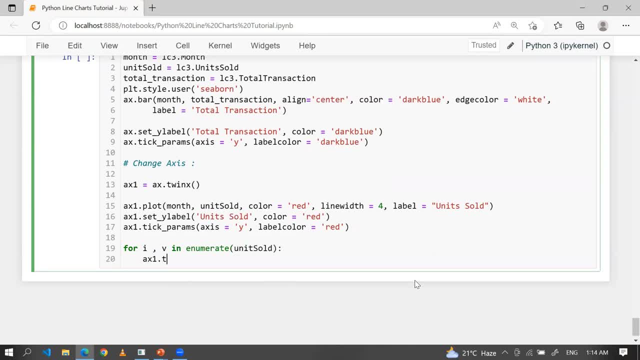 so for I and V in enumerator, and I want so for I and V in enumerator. and I want unit sold and here text color equal to unit sold and here text color equal to unit sold and here text color equal to red edge. so, guys, if you will create these, 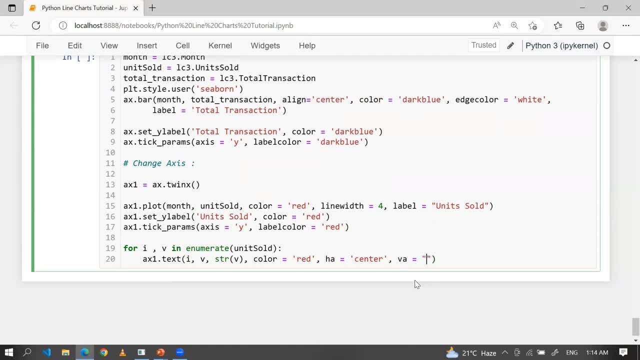 red edge. so, guys, if you will create these red edge, so, guys, if you will create these kind of chart multiple times right, kind of chart multiple times right, kind of chart multiple times right, so what will happen, you can easily so what will happen, you can easily so what will happen, you can easily remember these parameter for the long. 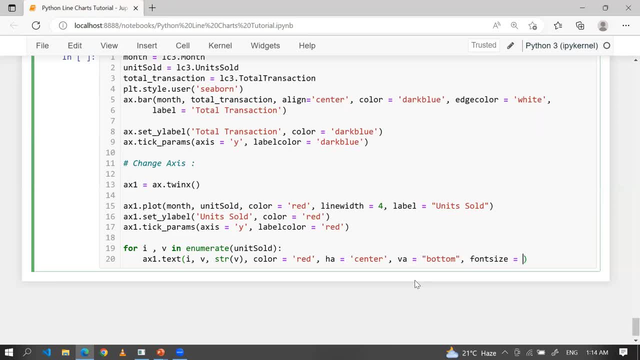 remember these parameter for the long. remember these parameter for the long time. it is completely depend upon how time it is completely depend upon how time. it is completely depend upon how you are doing the practice. okay, so font, you are doing the practice. okay, so font, you are doing the practice. okay, so font size: you can give. small you can give. 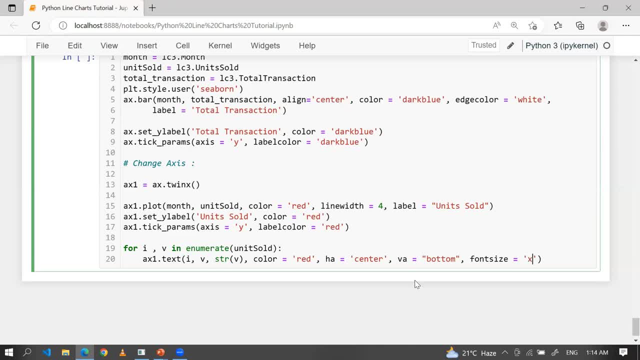 size. you can give small, you can give size, you can give small, you can give medium, you can give large, you can give medium. you can give large, you can give medium, you can give large, you can give extra large. or you can give X- no large, extra large, or you can give X- no large. 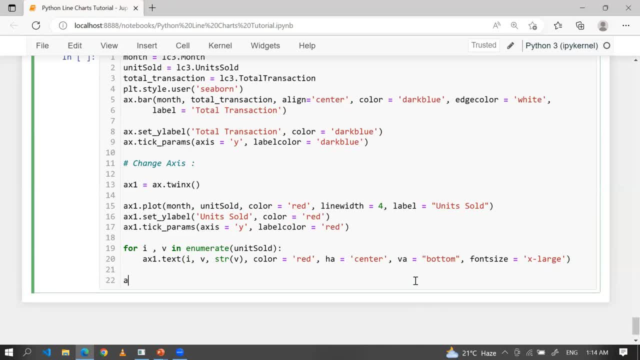 extra large. or you can give X no large, as in: and here X is dot lessened. let's as in: and here X is dot lessened. let's as in: and here X is dot lessened. let's say upper left axis one, not here one. say upper left axis one, not here one. 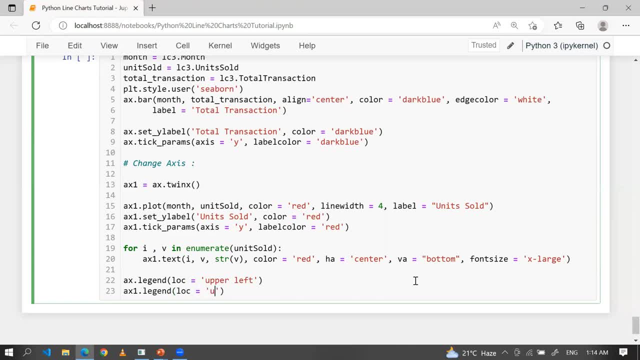 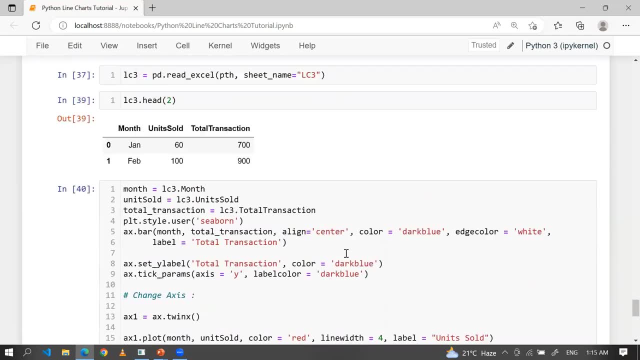 say upper left axis one, not here one. lessened lock equal to upper right. lessened lock equal to upper right. lessened lock equal to upper right. now PLT dot show. let me run this. okay, now PLT dot show. let me run this. okay. now PLT dot show. let me run this, okay, okay. so let me check the style guys. 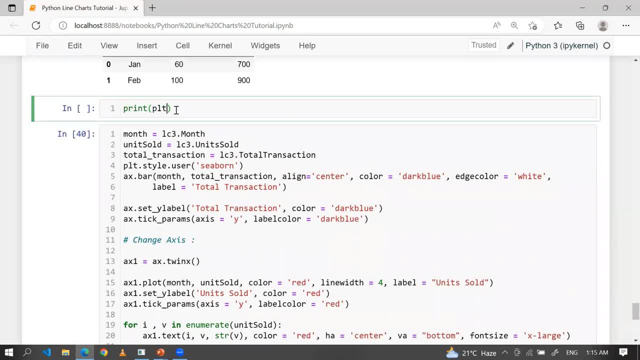 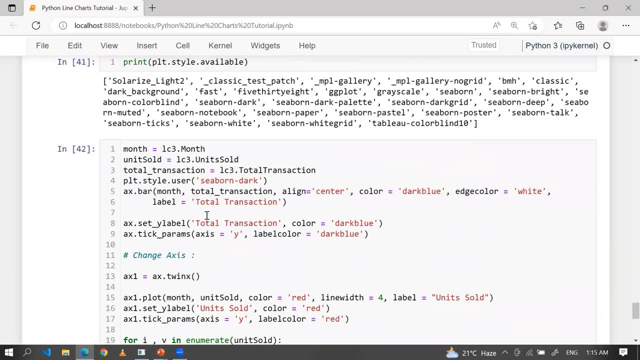 okay, so let me check the style guys. okay, so let me check the style guys again. so simple: print PLT dot style dot. again so simple: print PLT dot style dot again so simple: print PLT dot style dot available. PLT dot style dot. you sorry, 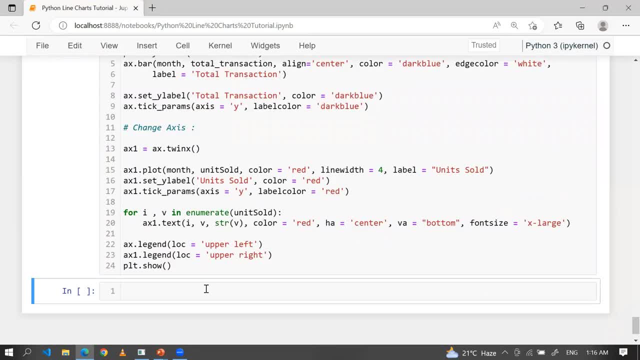 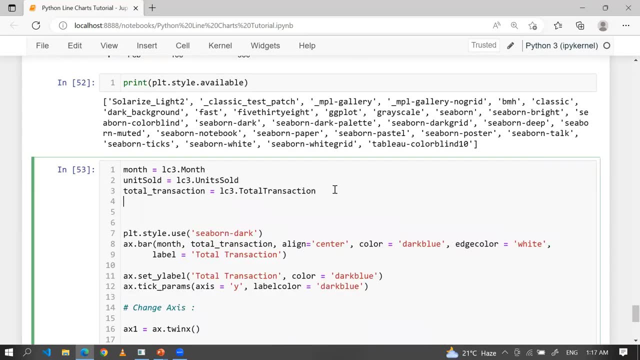 available. PLT dot style dot you sorry available PLT dot style dot you sorry not. user is a use PLT dot. show why it not. user is a use PLT dot. show why it not. user is a use PLT dot. show why it is not working. 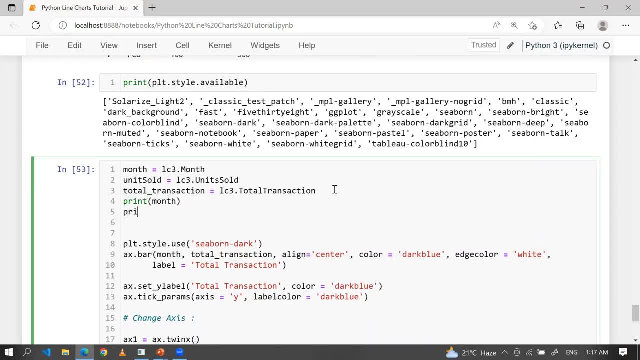 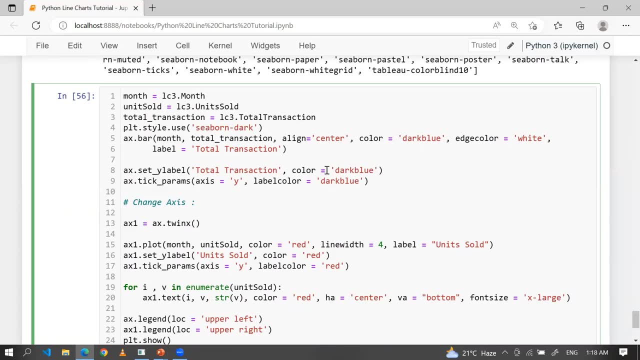 is not working is not working. let me print the month as well and unit. let me print the month as well and unit. let me print the month as well and unit sold and print total transaction. okay, so sold and print total transaction. okay, so sold and print total transaction. okay, so now let me run this. so, guys, we are why. 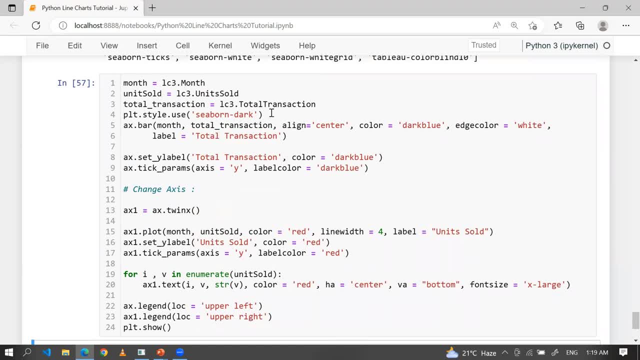 now let me run this. so, guys, we are. why? now let me run this. so, guys, we are. why we are not getting anything. X and X is: we are not getting anything. X and X is: we are not getting anything. X and X is Y. okay, so we, we haven't create the figure. 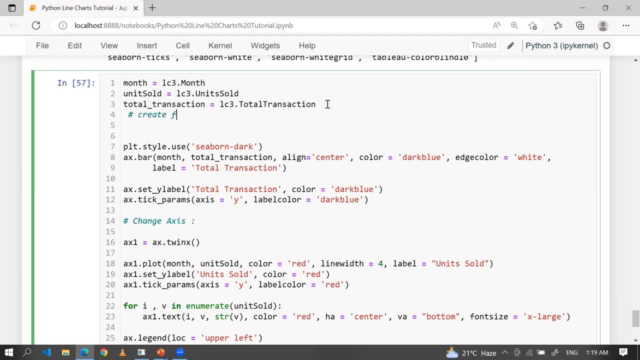 Y. okay, so we, we haven't create the figure Y. okay, so we we haven't create the figure and axis. okay, so now let me create and axis. okay, so now let me create and axis. okay, so now let me create here figure and axis- objects. okay, so how? 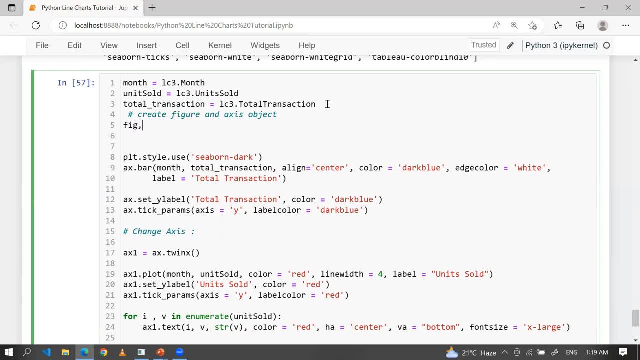 here figure and axis objects: okay. so how? here figure and axis objects: okay. so how we can create so simple fake, fake. and we can create so simple fake, fake. and we can create so simple fake, fake. and axis equal to PLT dot subplots. and here: axis equal to PLT dot subplots. and here: 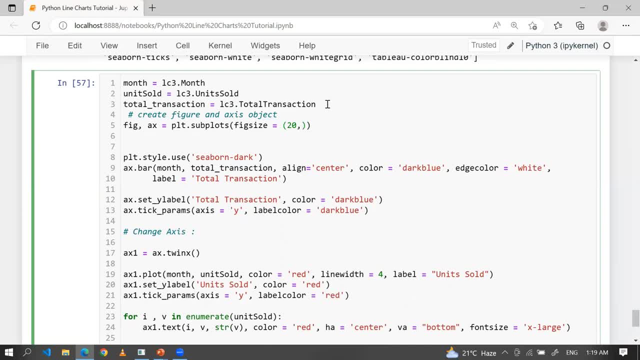 axis equal to PLT dot subplots and here big size equal to 20 by 7. okay, now, let big size equal to 20 by 7. okay, now, let big size equal to 20 by 7. okay now, let me run this. so, guys, you can see here. so 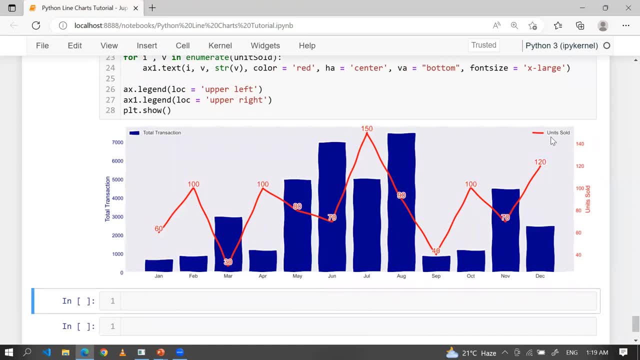 me run this. so, guys, you can see here. so me run this. so, guys, you can see here. so look at this. here we are getting the look at this, here we are getting the look at this. here we are getting the total transaction, and here we are getting. 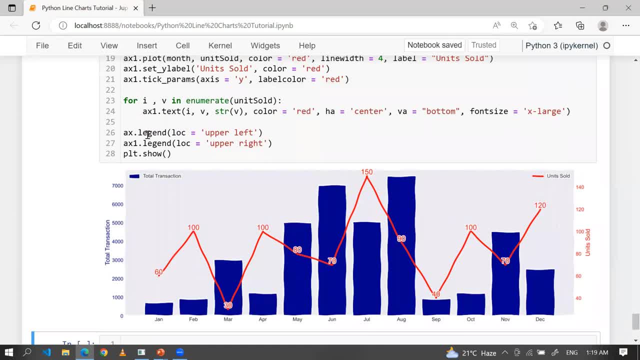 total transaction. and here we are getting total transaction. and here we are getting a unit sold. okay, so X is legend. a unit sold. okay, so X is legend. a unit sold. okay, so X is legend. right, so this is for the column chart and I. right, so this is for the column chart and I. 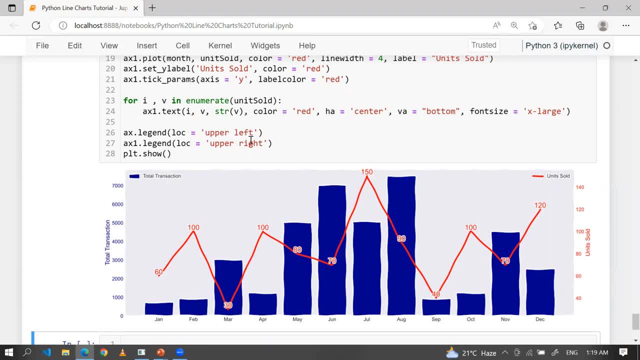 right. so this is for the column chart and I am going to represent is the upper am going to represent is the upper am going to represent is the upper. left axis one is the line chart and I am. left axis one is the line chart and I am. 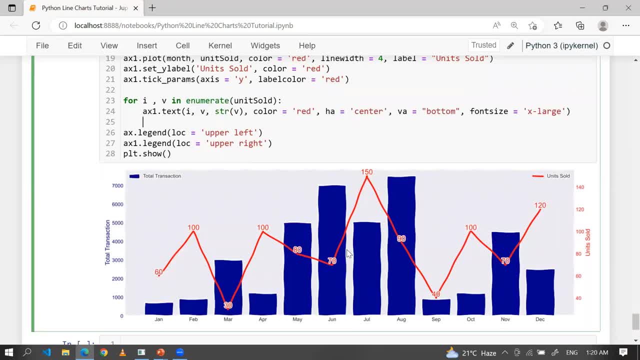 left axis. one is the line chart and I am going to represent as a upper right. okay, going to represent as a upper right, okay, going to represent as a upper right, okay. so, guys, here, I don't want the data. so, guys, here, I don't want the data. 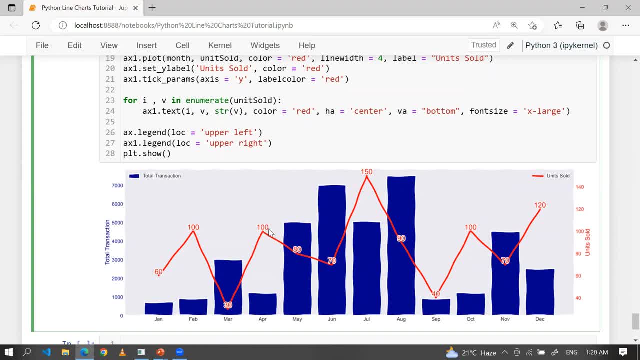 so, guys here, I don't want the data labels on the columns, I want the data labels on the columns. I want the data labels on the columns. I want the data labels on the line chart. so that's why I labels on the line chart. so that's why I. 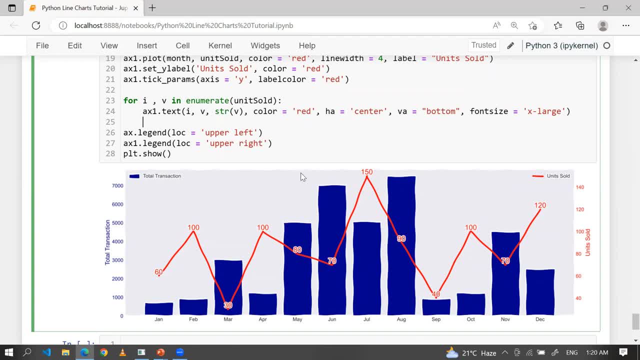 labels on the line chart. so that's why I have applied a loop on unit sold in, have applied a loop on unit sold in, have applied a loop on unit sold in case you want to add the data labels on. case you want to add the data labels on. 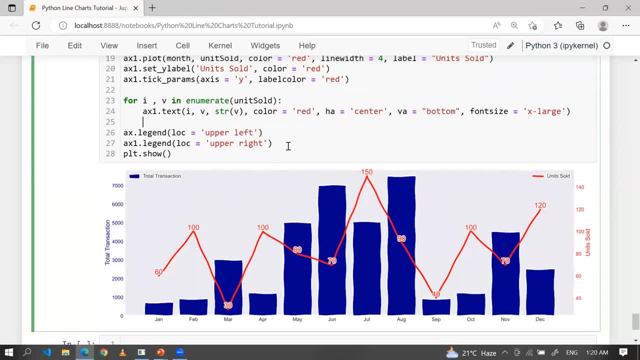 case, you want to add the data labels on total transaction. similarly, you can total transaction. similarly, you can total transaction. similarly, you can apply another loop for the same- okay. and apply another loop for the same- okay. and apply another loop for the same- okay. and one more thing on that: the ticks params. 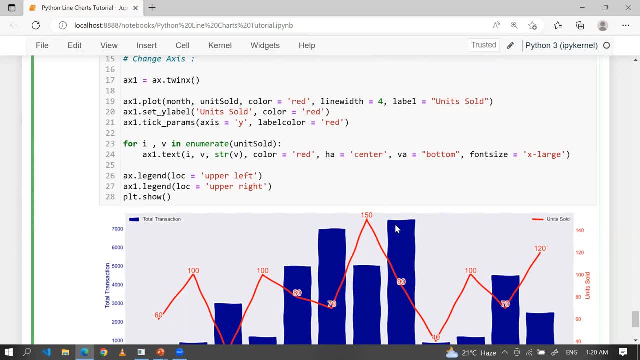 one more thing on that: the ticks params. one more thing on that: the ticks params right. so I want to, you know, change the right. so I want to, you know, change the right. so I want to, you know, change the data labels, or you know. or the colors. 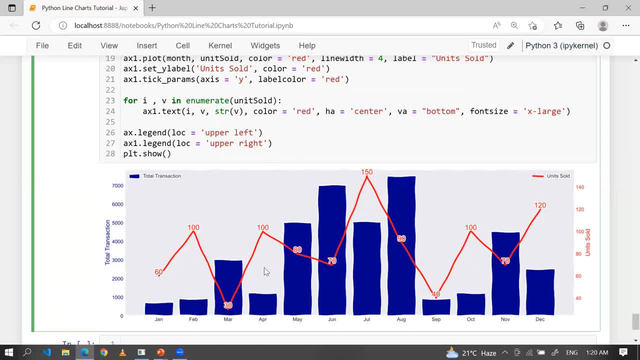 data labels or you know, or the colors data labels or you know, or the colors: the red on y-axis, so I have supply you the red on y-axis, so I have supply you the red on y-axis, so I have supply, you know, this color. similarly, I want to 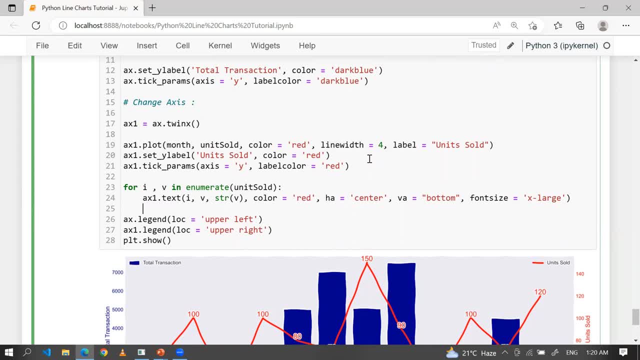 know this color similarly. I want to know this color similarly. I want to change my color on you know as a dark change, my color on you know as a dark change, my color on you know as a dark blue. so I have supply the dark blue as blue. so I have supply the dark blue as. 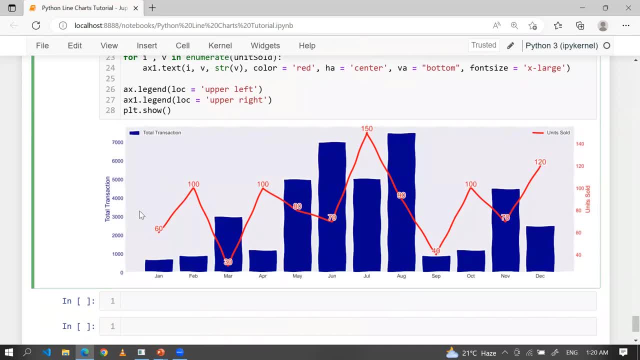 blue, so I have supply the dark blue as well. okay, so this particular part guys. well, okay, so this particular part guys. well, okay, so this particular part, guys, you have to keep in mind. all right, so you have to keep in mind. all right, so you have to keep in mind. all right. so, guys, again, a line chart is a chart. 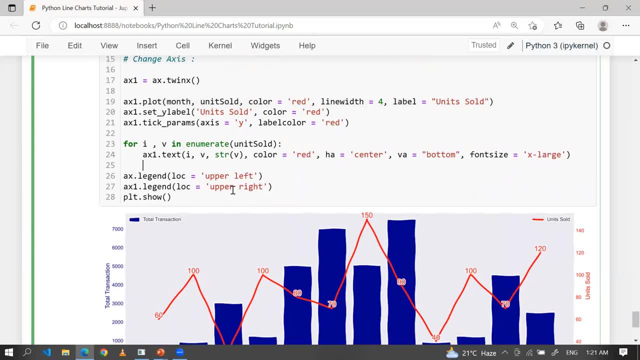 guys, again, a line chart is a chart. guys, again, a line chart is a chart. right that uses one of several line to right that uses one of several line to show patterns in the data. in case you want to show the patterns right, let's say how your sale. 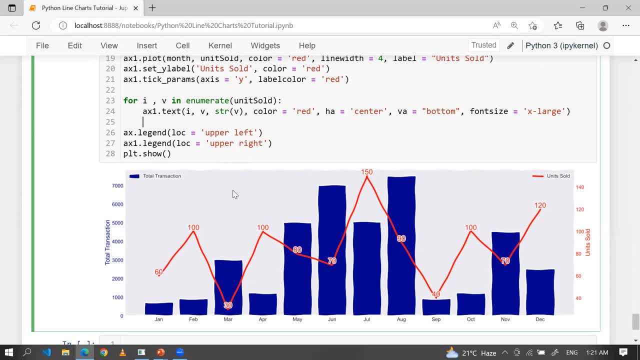 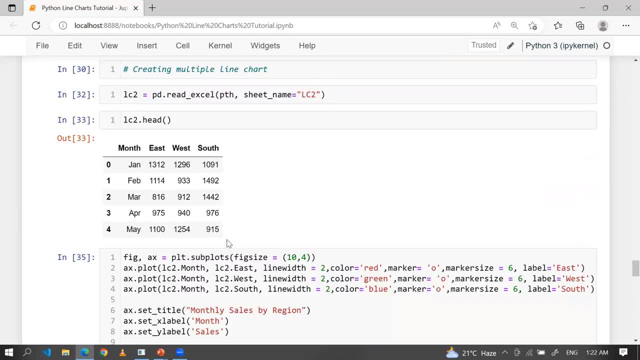 is fluctuating how your team performance is going on. in this scenario, you can use the line chart okay. so i hope you have learned a lot of things about the line chart in greater details. i have used several styles and plots with different, different mechanism with different, different. 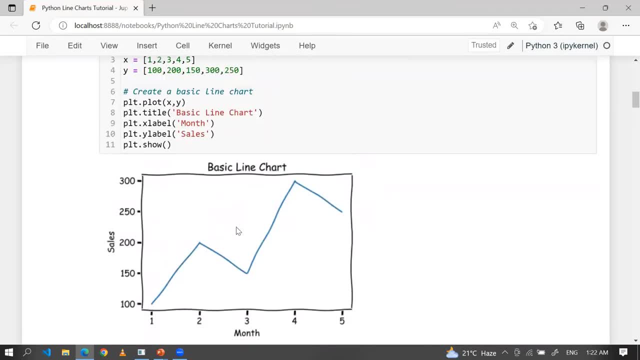 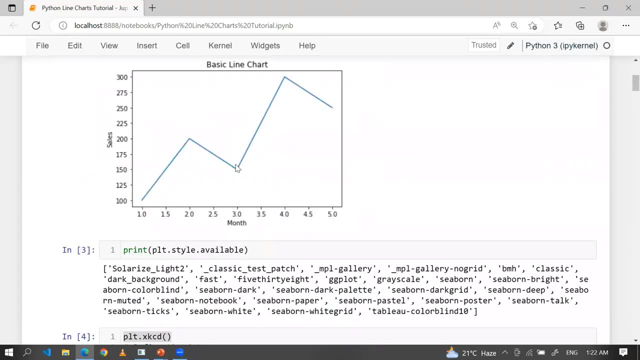 data set. okay guys, so please practice of this session and in case you are finding some difficulties, then please let me know in the comment and i will give you the link of this particular jupiter notebook and you can download and you can play with this around this particular stuff, whatever. 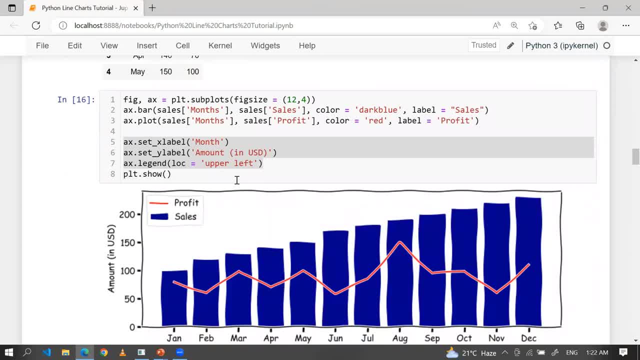 i have done it all right, guys, but again i am repeating myself: do the practice as much as you can, all right now, guys. i will meet you in the next session with some different set of agenda. meanwhile, do the practice of this session as much as you can and have a great day. bye. 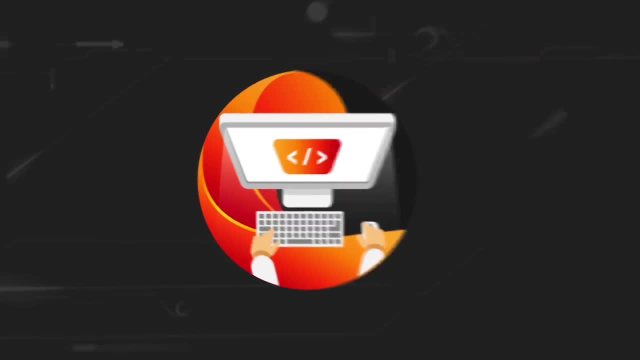 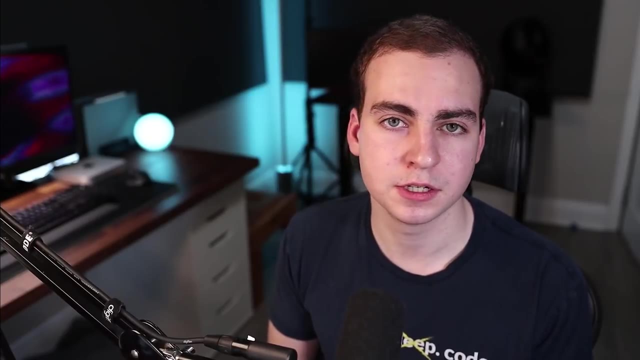 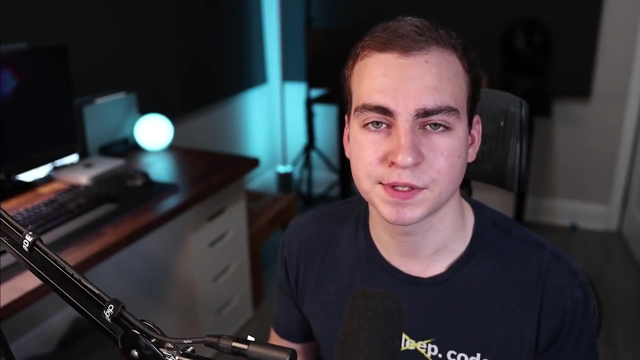 In this video I'm going to explain to you big O notation as well as how to perform time complexity analysis on various algorithms. Now I have a ton of examples and I want to make this video really focused on going through different examples and practicing performing time complexity. 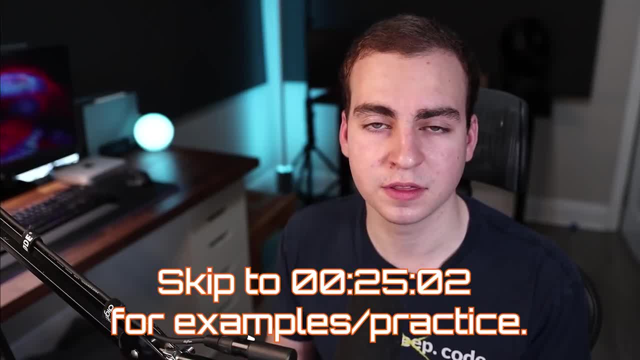 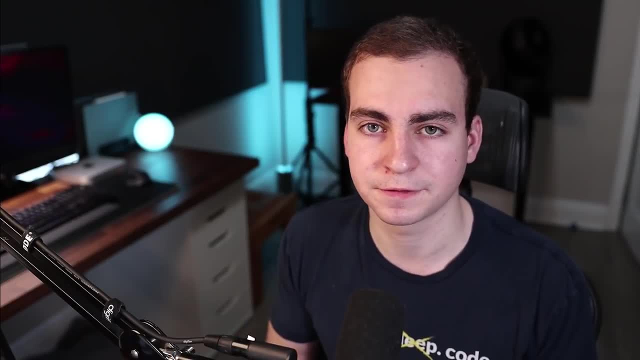 analysis. So if you're familiar with big O notation, skip forward in the video to those examples. They'll be in the video player or in the description. If you're unfamiliar with big O notation, then stick around for the first few minutes where I give you a conceptual overview.